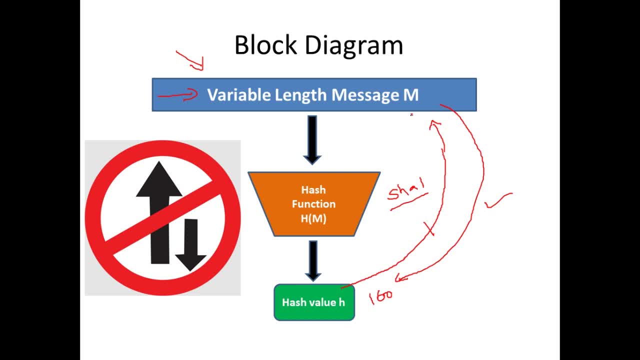 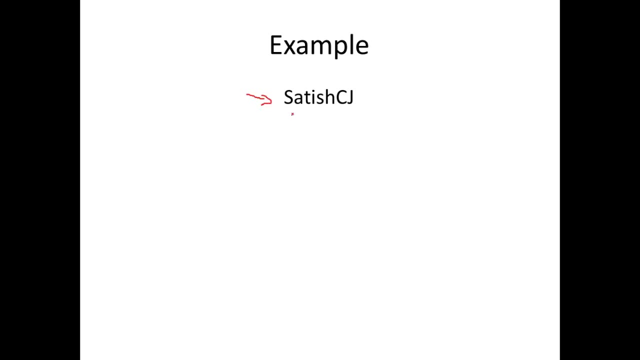 should never be able to get back the original message. So that's why we say these are one-way functions. This way is not allowed. Let's take an example here. For instance, if I give the input as my name, Satish CJ, To this hash function and say I've taken one sample hash function, sha1, and the output will be something: 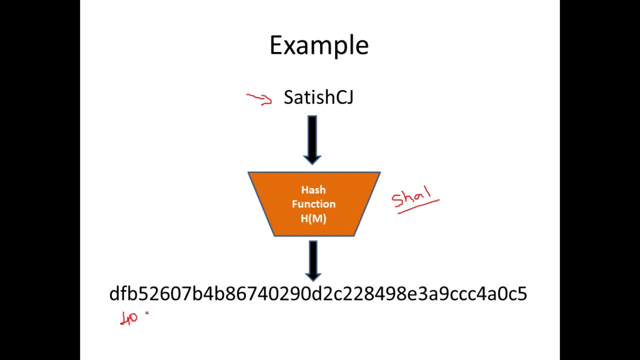 like this: So this is nothing but a 40 length, 40 character length hexadecimal value. or we can say, when you have 40 hexadecimal digits it's going to be 160 bit output, So you're going to get it hashed out. So this is the input. m. m is nothing but the text that is given as input. And let's take another. 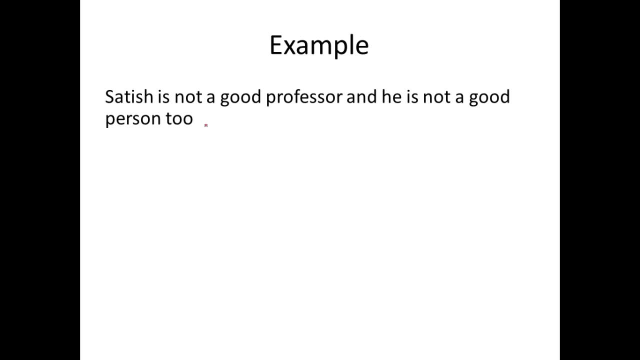 example, Let's say Satish is not a good professor and he's not a good person too. So now, this is the text m and you. now you see there is a variable length. In the last slide we add this to be the input, Whereas in this the length is varying and we give this to our hash function. Say again, we: 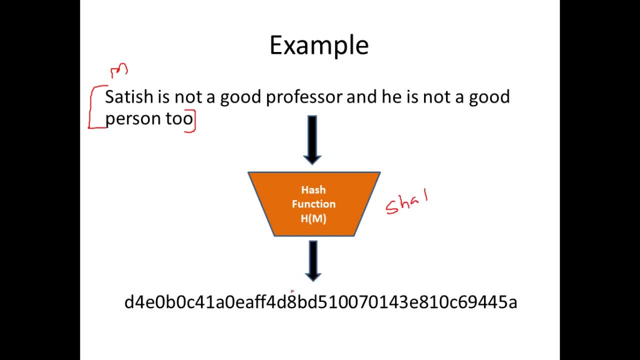 give it to hash function sha1.. The output here will be the input m. m is nothing but the text that is given as input. So this is again an hash value with 40 hexadecimal characters or 160 bits. So what we understand from here is: no matter what is the size of the input, the output will always be fixed. 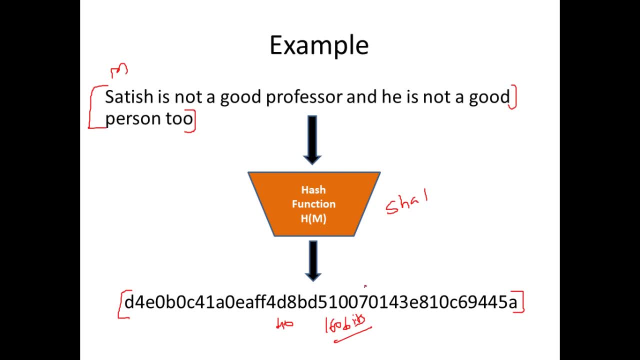 like 160 bits or 40 hexadecimal characters when you're going to use sha1.. But if you use another, if you're going to use some other hash function, the output fixed length can vary. The length of the output can vary. Say, if I use some other hash function, the output fixed length can vary. The length of the output can vary. Say, if I use some other hash. 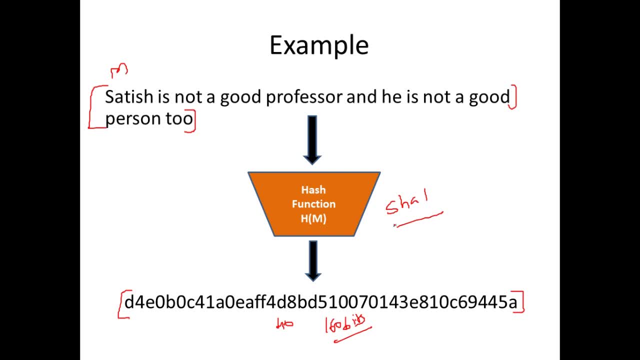 function. the output can vary, but it will be of fixed size. When I use sha1, the output will always be 160 bits and that is the hash value. And another important thing we have understood is: using this hash value, I will never be able to. 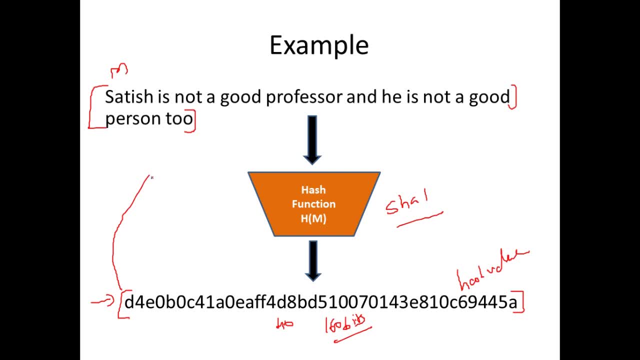 again track back to this original message. So there is no way I can take this hash value, just this hash value, and then find out what is the original message that it is corresponding to. So it's not like encryption and decryption. In encryption and decryption we used to encrypt something, a plain. 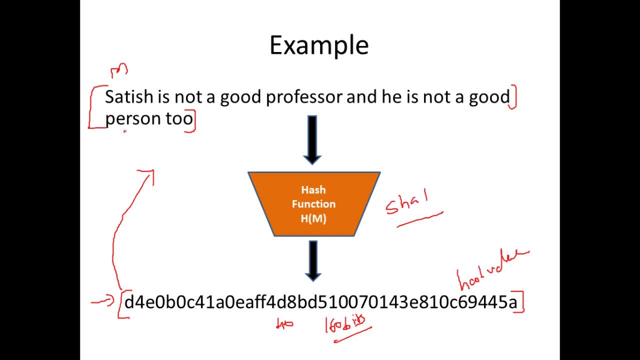 text will be encrypted. Likewise, after the receiver receives it, you will be able to decrypt it, decode it back to the plain text, Whereas here there is no such thing. if you get the hash value, you will not be able to get the plain text back. That is the key difference here. 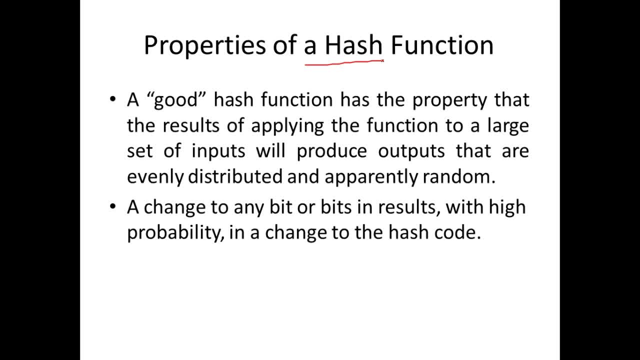 So let's look at the properties of a good hash function. What do you mean by a good hash function? So a good hash function should lead us to evenly distributed and random outputs. So for a message that's coming in, we should get a random output. 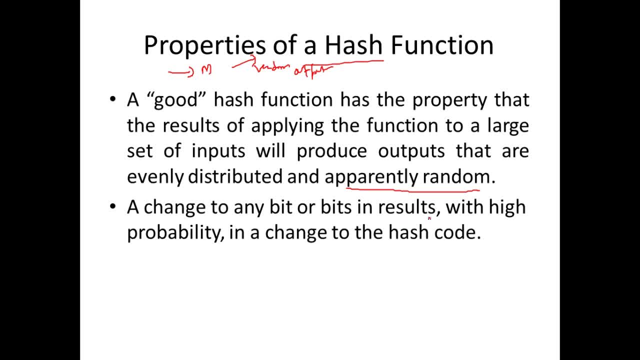 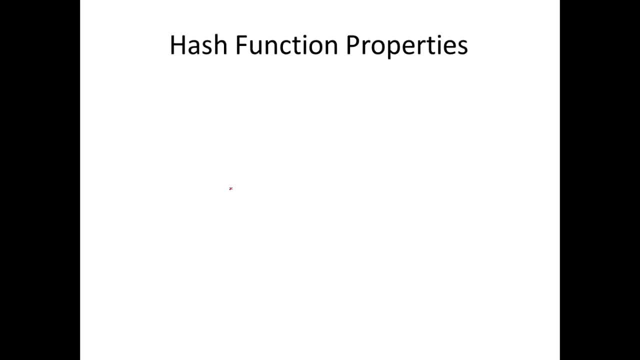 And a change to any bit or bit bits results with a high probability in change to the hash code. We'll understand these two things with a visualization. So for the answer to this question we need some sort of a hash function. so I have this. my name is given as an. 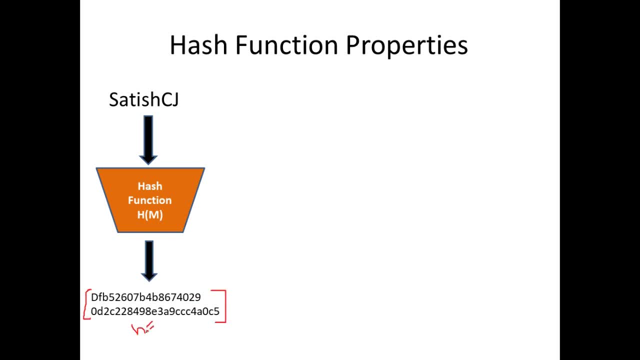 input to this hash function and the output is a 40 digit hexadecimal character. This is what we are seeing, this is the hash value h. and if I give a totally a different input, say professor, and if I pass it to this same hash function, partner primo, et cetera, et cetera, and so forth, statut. So if I consider all the hash function="http 8: 2012.2.3.10. Haven- Provider: 0 means 1.4. Harris hh gak prime, 1.5.. Part 1: double attack: 304.1.0.12.0.�� r d Doctor Golden: 0 i no 4, 0.088.11.0.3.10. 1985: 0 sense 01. So I give a totally different input to this hash function and the output is 40 digit hexadecimal and. 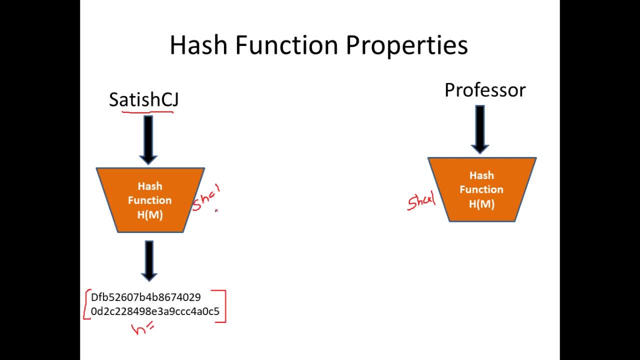 consider all the hash functions or SHA1. here We take the same hash function and give a different input, Then obviously this output should be different from this output. So two different inputs should give us two randomly or two different outputs, And there is one. 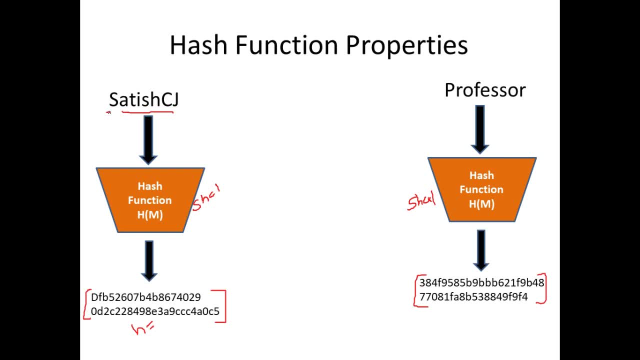 more thing that we have to understand. Suppose, if I change a single character here or if I do make some small changes, say, this is changed to a lower case, this s is changed to a lower case, And if I pass it to the same hash function, SHA1, the output you see here. 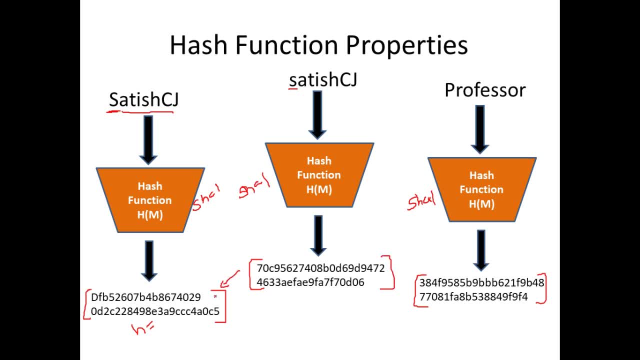 this output is totally different from this output. So, though there is a very small change that leads to a major change in your hash value. So this is called the avalanche effect. Even if I change one bit or a set of bits, the output should be totally different from what is that we got. 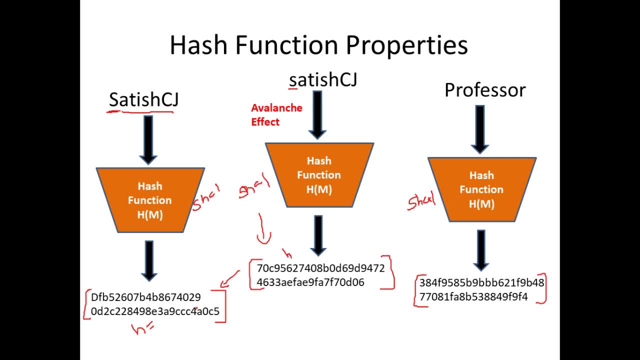 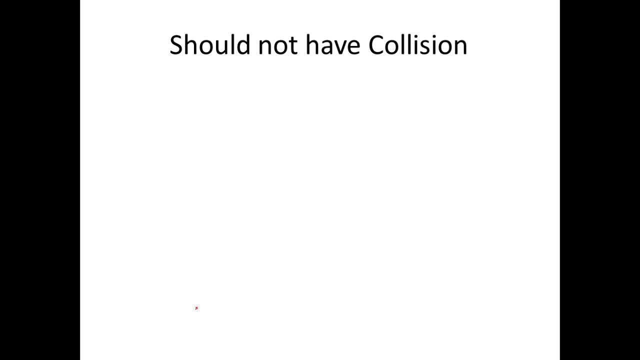 before changing the input. So these are some properties of a good hash function And we have to understand this should not have collision. Most of you might be knowing what is collision resistance. You would have learned hash functions in your data structures and databases classes. 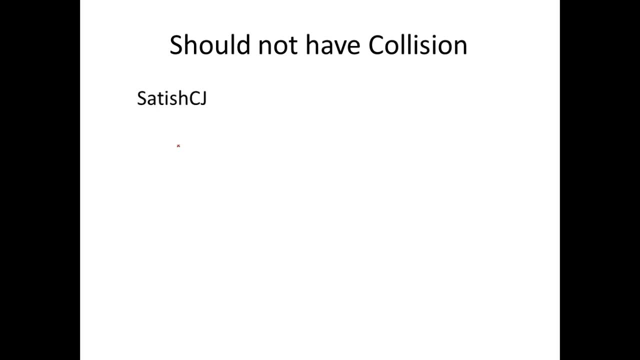 But let's take a look at collision. What does this collision mean? Say, if I have this input, satish cj, and I give it to a hash function as usual, let's say this hash function is SHA1. And what will be the output? I'll be getting a 40 digit hexadecimal character. 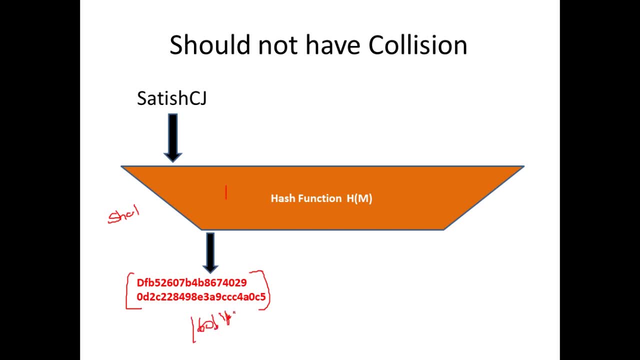 or 160 bits. So that is there. Let's assume that I'm giving a totally different value. It's just an assumption here, And I'm passing it to the same hash function, SHA1.. And if, by chance, I'm telling you, by chance, I'm giving you by chance, by chance, by chance. 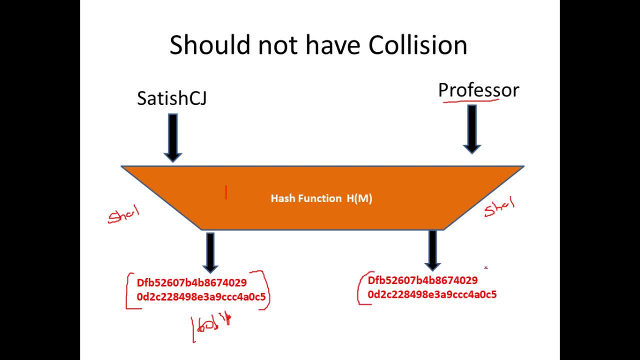 I'm telling you by chance. I'm telling you by chance. I'm telling you by chance, I'm telling chance, if I'm going to get an hash value which is exactly the same as this hash value, say, the inputs are different, but then the hash values somehow come out to. 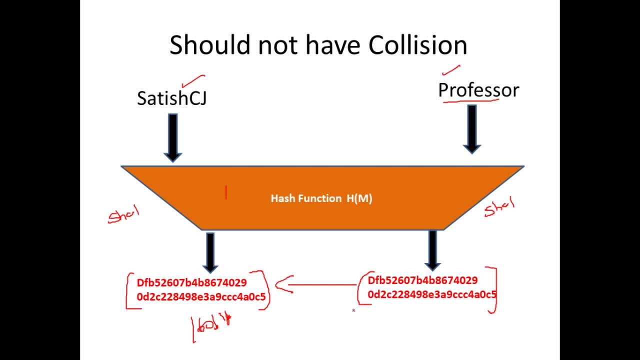 be the same. that can happen. so in that case we say that is a collision. so you should never get the same hash value for different inputs. that is not a good hash function, so we call that to be collision. a good hash function should be collision-resistant or it should give us very random outputs and that is. 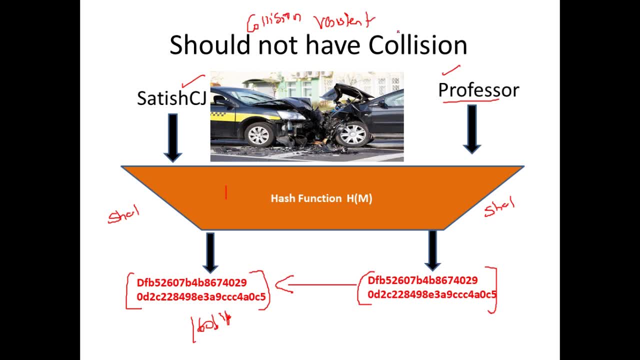 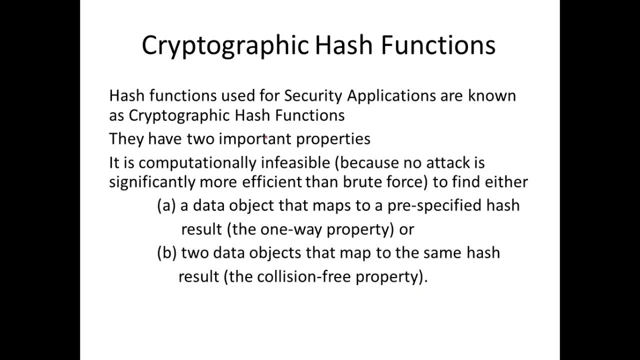 evenly distributed, okay, so please keep this in mind. collision is not good for an hash function. now let us take a look at cryptographic hash function. so when I say cryptographic hash functions, what are the most important properties for hash functions that are used in cryptography for security reasons? so here the two important thing is: only brute-force attack can, should be. 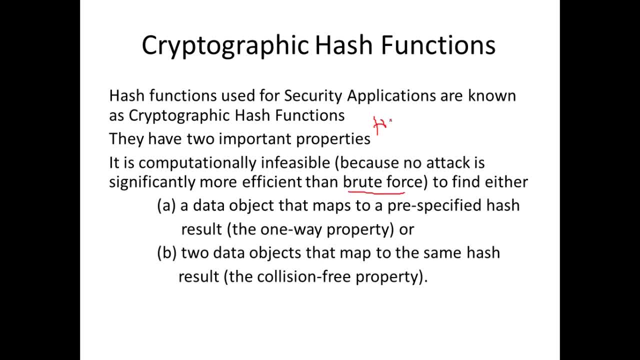 able to crack it. for instance, if I use an hash function, H of M, and I get a value H, say let's take H of Satish, let's take a simple example here and say: this is hash, something like this: a F, 2, 3. so this is the hash value. 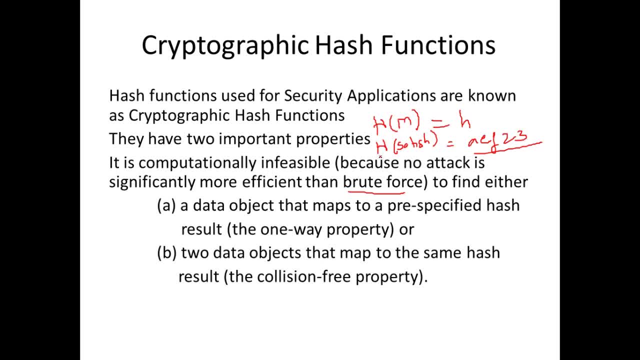 so if you're going to use this in cryptography, the key concept is: if one hacker gets to know of your hash value- say, some hacker gets to know of this hash value- the only way you'll be able to find this is corresponding to satish's. you should be going with brute-force, that is, you should take every word, say: 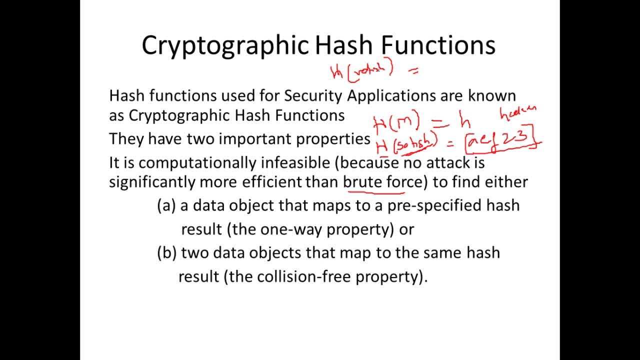 H of Ratesh. so this is capital H, H of Ratesh. he will get something like B, E, K, G, D. oh so I'm sorry, this is an hexadecimal right, so it should be B, E, A, 2, 4, 5, something like that. so again, these are. 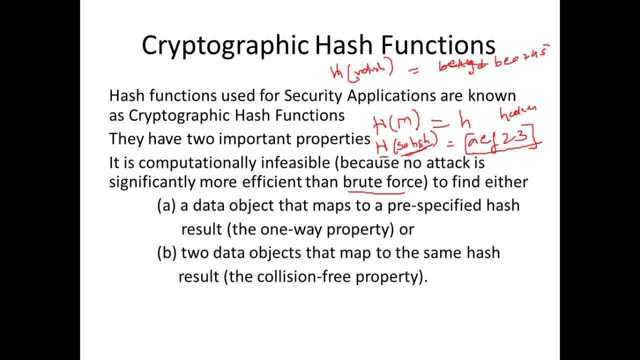 imaginary values not corresponding to any hash function. so you should just keep on checking all these input values to check where exactly this hash matches. so when that match will happen. only when he enters H of Ratesh by brute force, all the values he enters, and then he enters Ratesh. 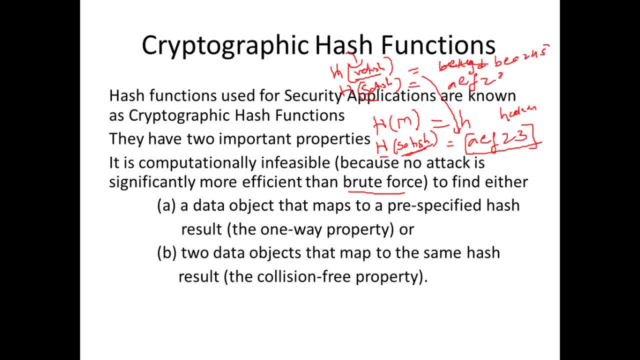 and then what he will be able to hash to: A E, F, 2, 3. so whenever you give Ratesh, the output will be A E F, 2, 3. so the hash value will be the same for the input, but for different inputs there will be. 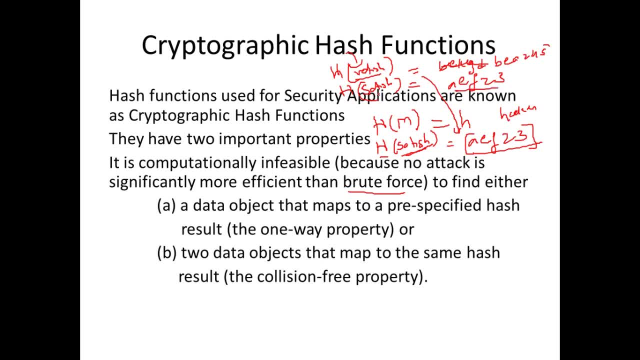 different hash values. so to find out what is the corresponding text to this hash value, he has to go with brute force. we should be able to crack a cryptographic hash function only using brute force. you know how difficult it is. just passing on all that text combinations on. 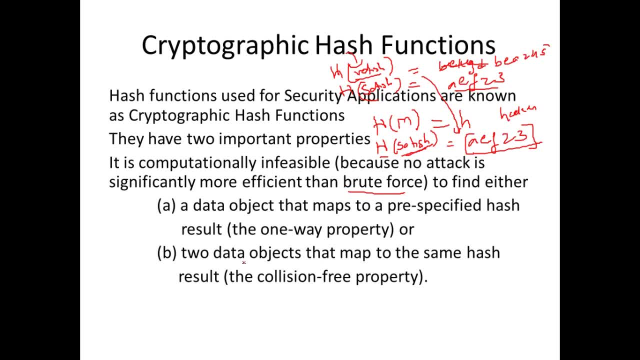 earth. it's not, it's not going to happen- and two objects that map to the same hash result, that is, collision free property and this also should be. you know, I'll just explain. you say, for instance, we have H of Ratesh. let's say there is this hash function, H of Ratesh. so this is: 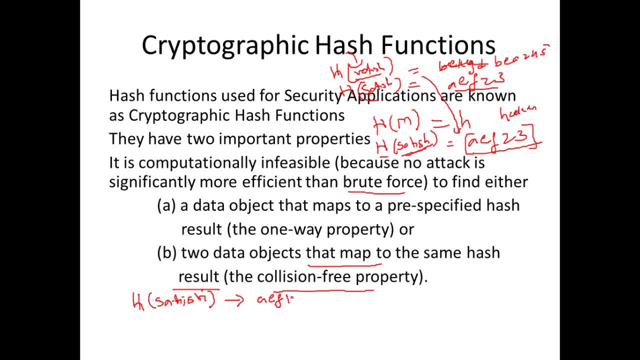 being hashed to a values. let's take A, E, F, 1, 2, 3, and there can be another. it's always possible that there can be another statement or another input message, say professor, or something that will also be able to hash to the same value. it's possible hash functions can lead to collision, but 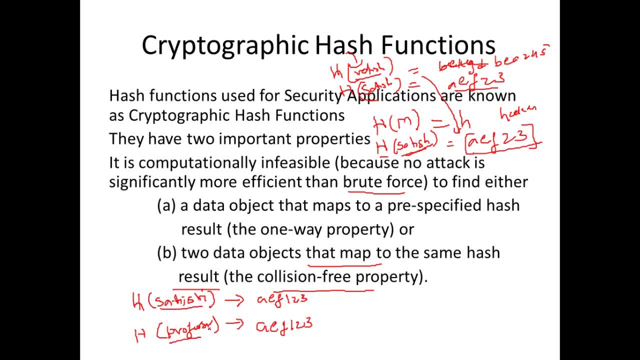 finding that Satish and professor have the same hash values. how an hacker can do that, it should be only through brute force. brute force in the sense you should take Satish, find it out, then you should take all the other words that is available to him. hash it out to check, okay. 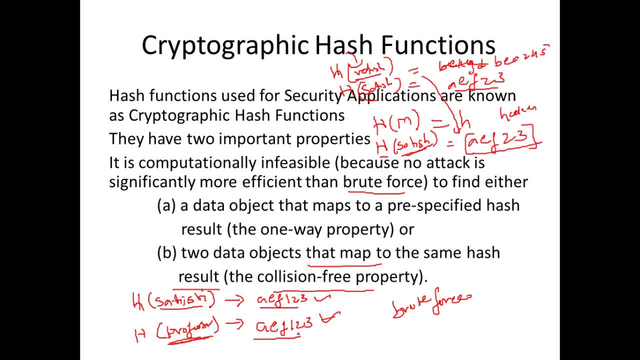 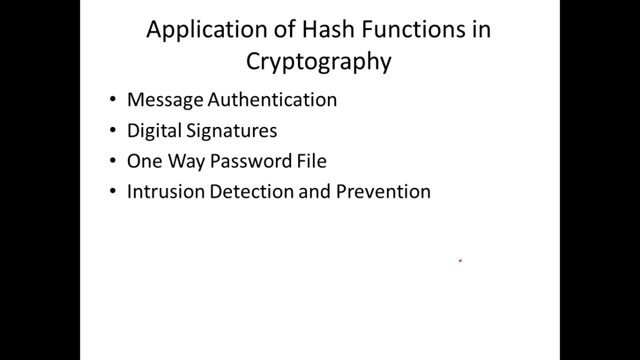 professor and Satish lead to the same hash value, so you should be able to detect collisions only using brute force. and why should a hacker even detect collisions? we'll understand that in the coming slides. now let us take a look at what are the application of hash functions in cryptography. we looked at what is. 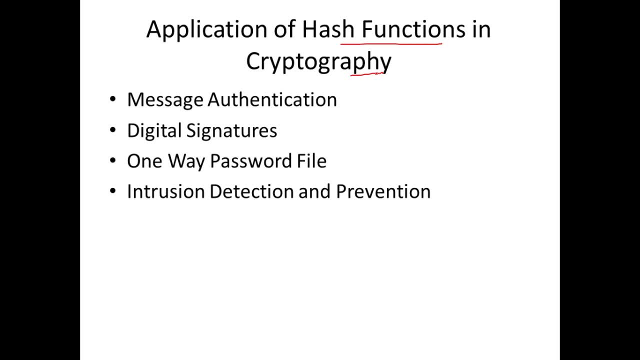 an hash function. we take text, we just convert it to a fixed bit output. we call that an hash value and we say these are one-way functions. we cannot take the hash value and find the input message. so what is the application of this in cryptography? we will use this in various places, like message. 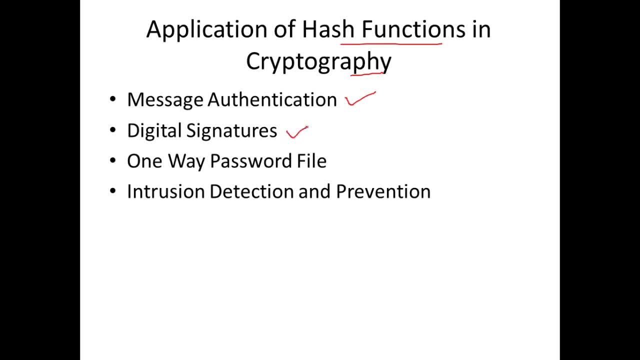 authentication. we'll use it. that for digital signatures. we'll use that in password protection in your databases also, we'll use password files and inclusion detection and virus prevention systems also use hash functions. so we look at all these things one by one now how it is used in message authentication. so message authentication is a. 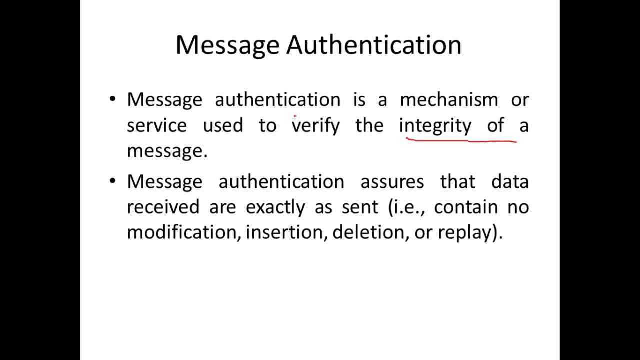 mechanism service used to verify the integrity of a message. so if somebody sends you some message, an email or a file, how will you know that you are receiving the original file that has been sent from the user? how will you ensure that there is no one who has really changed or modified, inserted or 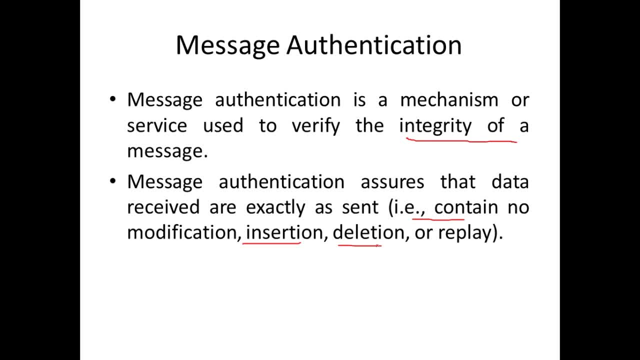 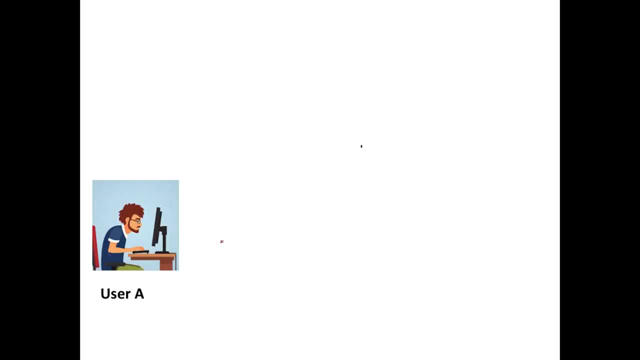 deleted contents in that file before it reached your destination. okay, let's understand this entire thing with an visualization. say, you have user A and the user A is communicating with user B and they are friends and they are communicating over an insecure channel. what I mean by an insecure channel? that is, you have a third party listening, maybe an hacker or 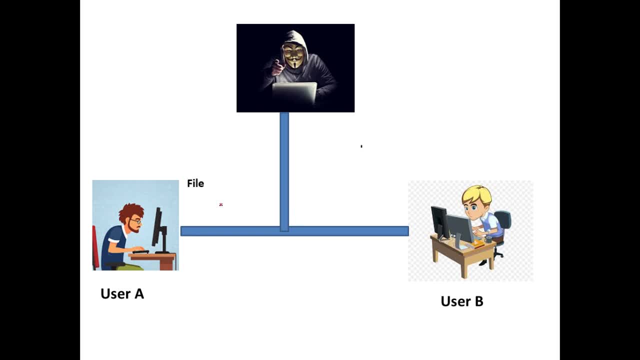 someone who is listening to the communication, and user A wants to transfer a file to user B and he is very concerned about his faculty, Satish, and he wants to help Satish. so this is the message inside this file and what he is going to do is he is going to send this file to user B. 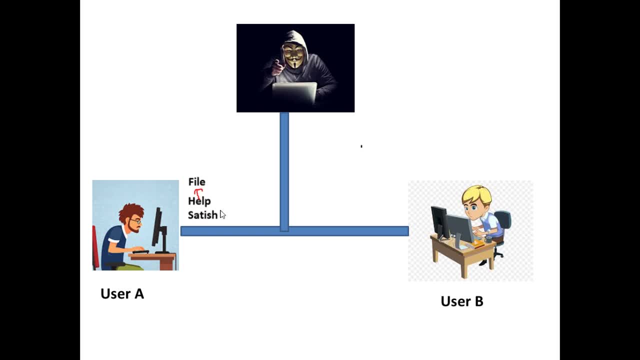 so he just wants to convey this file. so when he transits this file this hacker somehow catches hold of this file and then he changes the contents in the file. so he creates a file similar to what this guy has sent. but then he changes the input message along: instead of helping Satish, he says kill Satish. 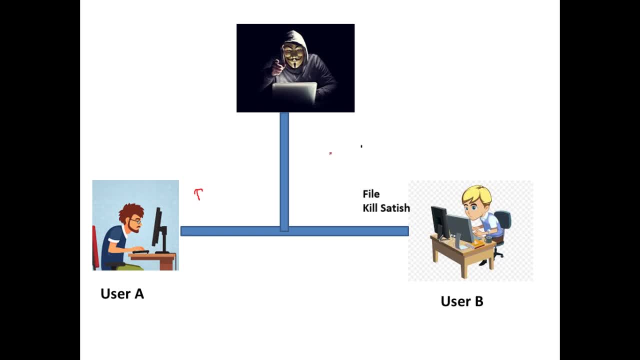 and he sends that file to user B. now this user will think that this file has come from user a and then is going to take the action as instructed by user a. so this action is extremely opposite. so is going to happen to our professor satish after this message reaches user b. so this is a problem. 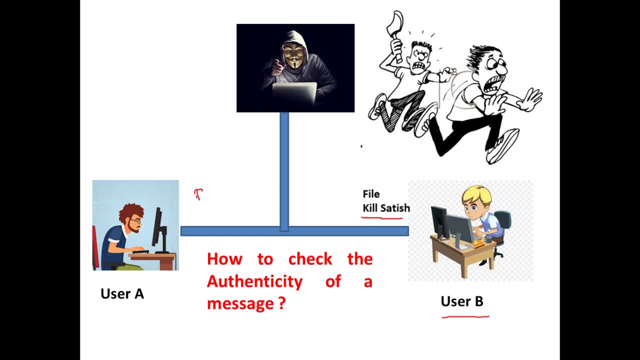 like how to check the authenticity of the message. you can. you can get a file, you can get a mail, you can get a message, anything from user you're communicating through an insecure channel, and how to ensure that nobody is intercepting your messages and they are not altering the messages. 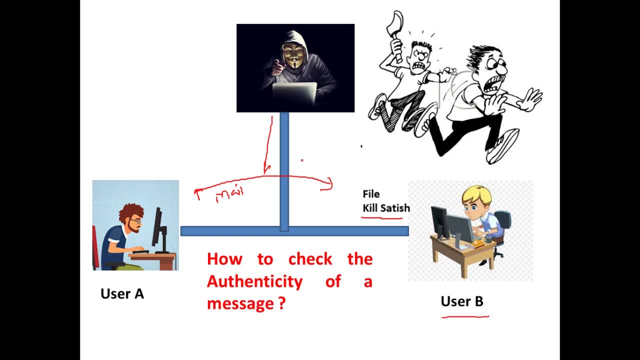 and you're just getting the original message. one first thing is: how's that you? we're going to check whether you're getting the original message, like that, and the next thing you have to check is: are you getting the message only from user a? how to know this? so these are the 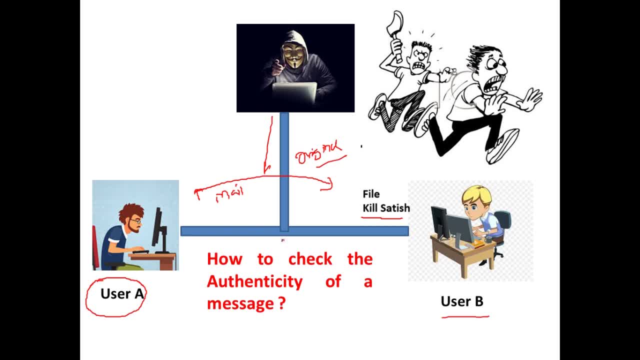 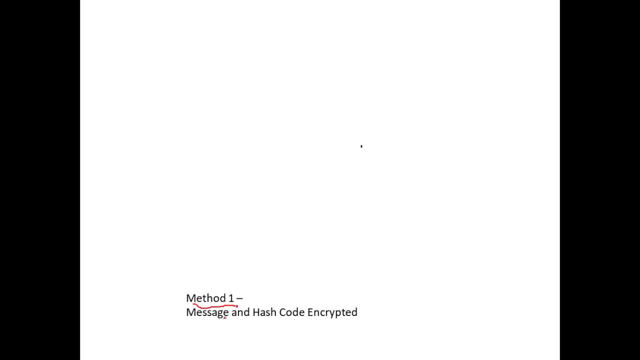 two things that is really bothering us, and for that we have hash functions helping us. let's see how. so let's take a look at method one: message and hash code encrypted. we'll see this method in. we'll understand how this particular method helps us with respect to 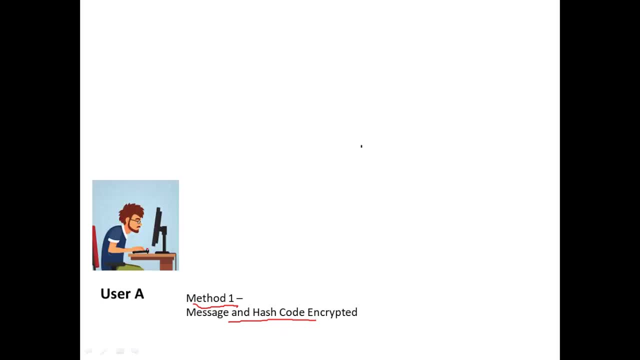 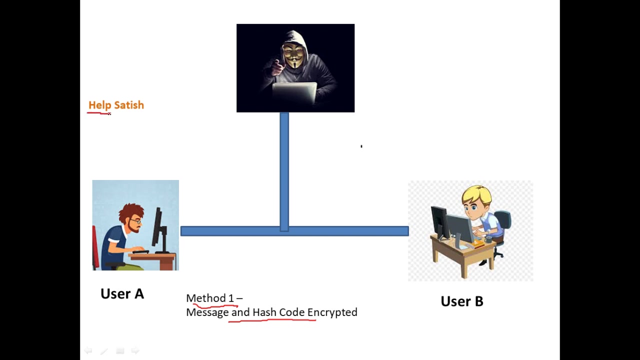 providing message authentication. so we again have user a and you have user b, and user a and user b will be communicating over an insecure channel and this hacker is listening to them. and again, this user wants to send this message in a file to user b. right, so what he will do is he will take. 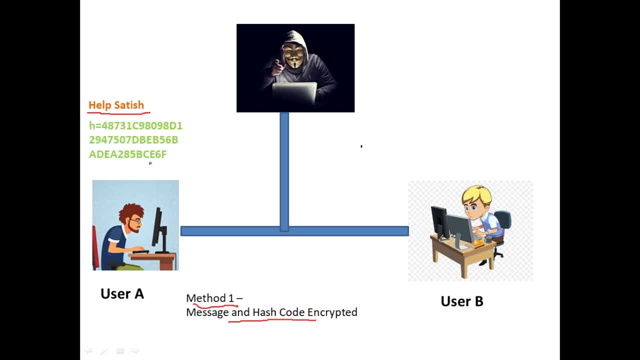 this message and he will send this message to user a and user b. right, so what he will do is he will take this message and then you will pass it to a hash function and hash it. so if this message is getting passed to an hash function like sha1 and this hash value is generated after generating this, what he is going? 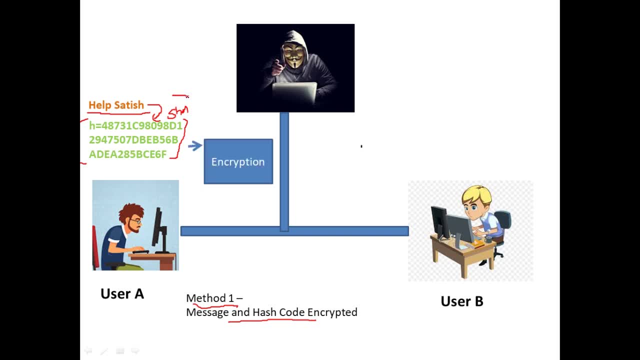 to do is he is going to take the message and the hash value and then he is going to encrypt it. encryption can be using aes encryption or any blocks like encryption. so symmetric key encryption is going to perform and then for that you'll be using a key for encryption. we have learned so. 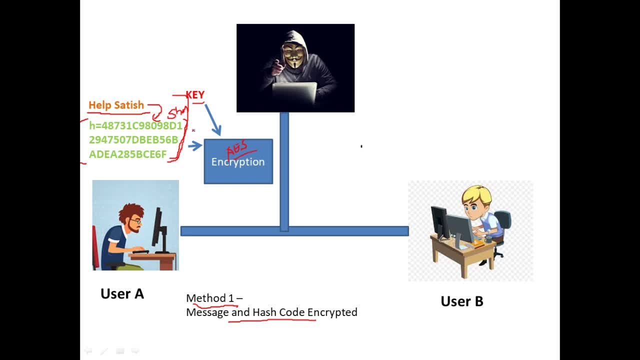 many different types of encryption. let's say he's using aes, so he encrypts this hash value and this text, and then he's going to get some cipher text right and then he's going to send this cipher text to the user b. now what user b is going to do is he is going to decrypt it. so again, aes decryption. 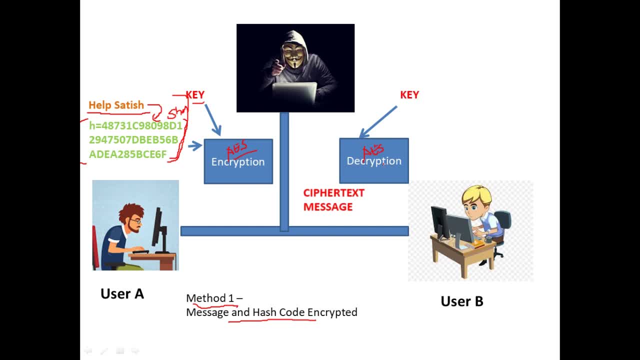 for that. he is going to use the key and he is going to decrypt it. when you decrypt it, what he is going to get is going to get the text message along with the hash value. so you will take this text message and then you will compute the hash. so you will take this test message, give it to sha1 and then you will be computing the hash. 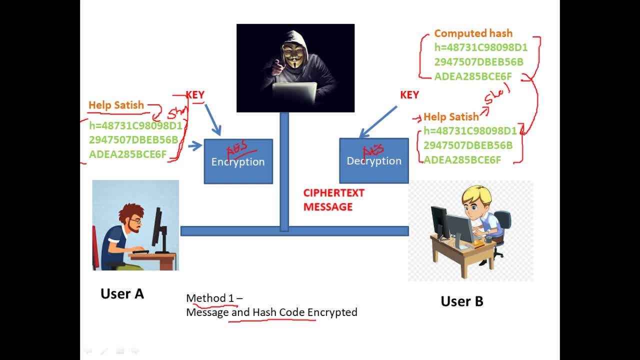 and then you will check whether this hash value matches the hash value that you have received. so only then you can understand that the text was not altered. so when will you use this when you want your message to be also very confidential, so this guy actually will not be able to read the message or the ash code, because everything is encrypted and 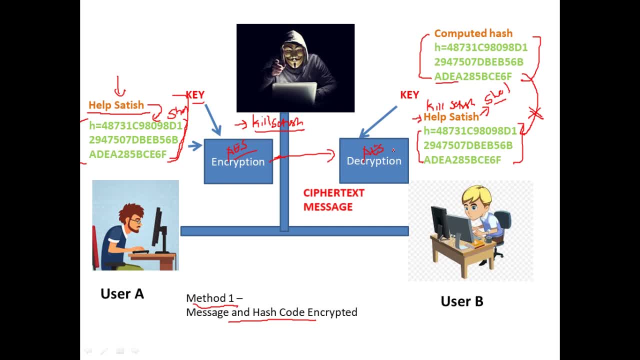 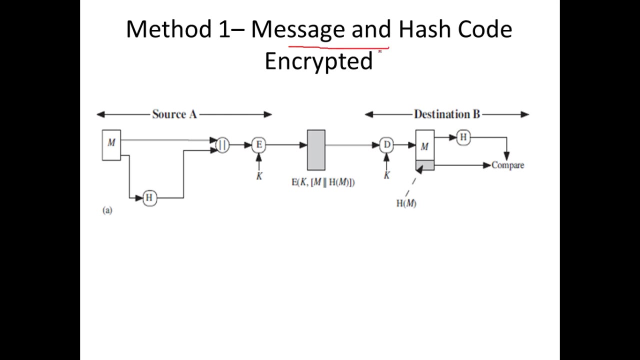 sent. so there itself the security comes into place, and we all know nobody has broken aes2 right, so hacker has no way of getting hold of the information here. so that is my visualization. when you take a look at your textbooks, they are given this kind of a. 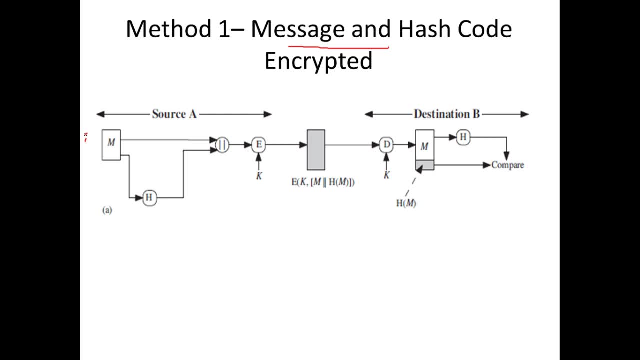 diagram. so this is the message sent by user a. let me write: user a is here, is sending this message, so what he does, he first hashes it, so h is the hash function, so h of m he does. and then, once when he hashes this message, what he does is this hash value, that 40 digit hash value. he. 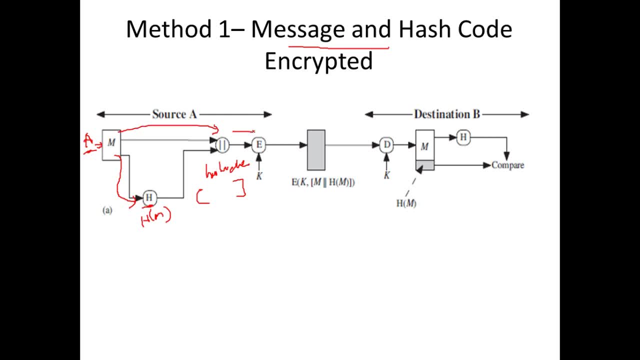 concatenates that with the message. so he helps satish and hash code is being encrypted with a key. this is where aes kind of a cipher- i mean block cipher- comes into place and he sends that and while the user b receives it, you will decrypt it again using aes. you will decrypt it using the key. 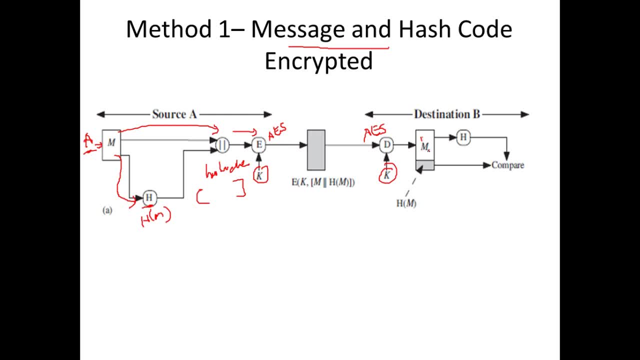 and that will lead us to what we will be getting: the message help satish. and the hash code h of m. so now this user will take this message. you will again use this hash function, like sha1, so you will be able to generate the hash code. you will compare that. okay, this is the hash code i. 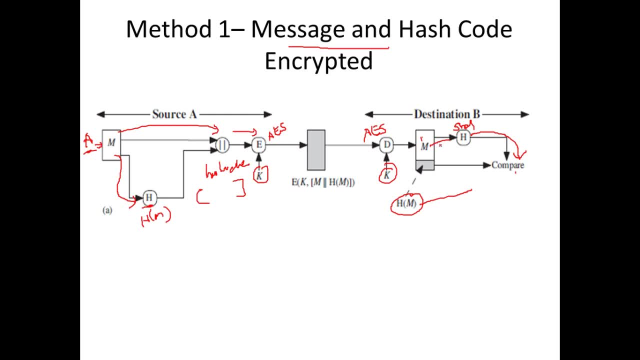 have received and when i encrypt the, when i hash the message, this is the hash code i am receiving. so are these two hashes the same? so when these two hashes are the same, then you can say yeah, then you can be sure of that. he has received the message sent by user. a right, let's take. 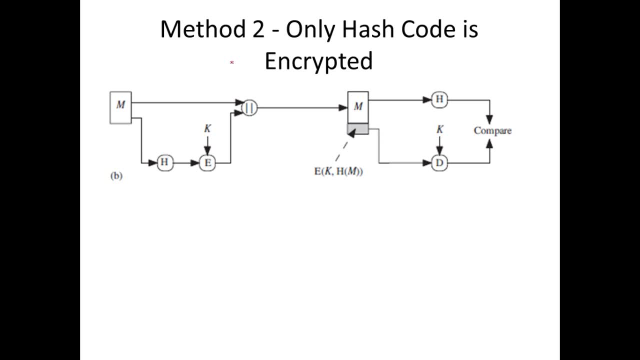 another method, method two. this is a slight uh variation from the previous method. here we are not encrypting, we are not encrypting the message. we may feel that the message is not so confidential, but it should not be altered uh during its weight on its way to the user's destination. so here we are not altering or we are not encrypting uh message m. 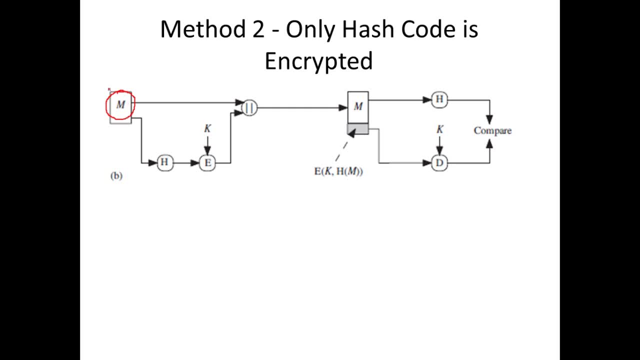 what we are doing is we are just encrypting the hash code. say, if message m is help satish, what we are doing here is we are taking the message m, we are converting it to a hash value. so h of help satish, that is h of m, we are. 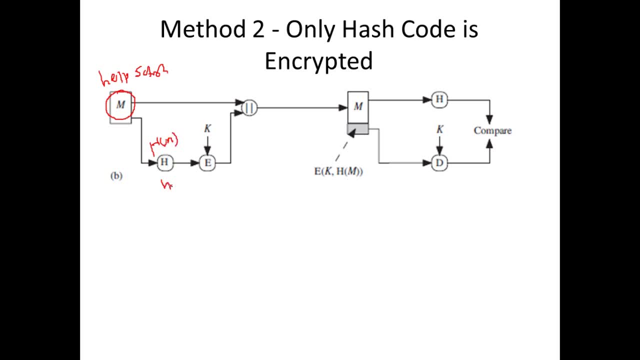 doing. we'll be getting this hash value h and then this hash value, this 40 digit hash value alone, we are encrypting. say, we'll use aes and a key to encrypt it. so this hash code alone we are encrypting. so we're just encrypting 40 digit input. we are just going to encrypt that and we are going to. 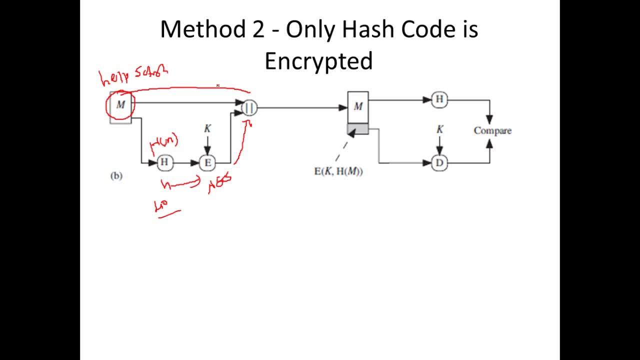 take this message: help satish concatenate that. so help satish is plain text. the hash code is encrypted and it is being sent. so what is being received? the plain text. help satish will be received here and help satish should be hashed. so he is going to get a 40 digit hash value. 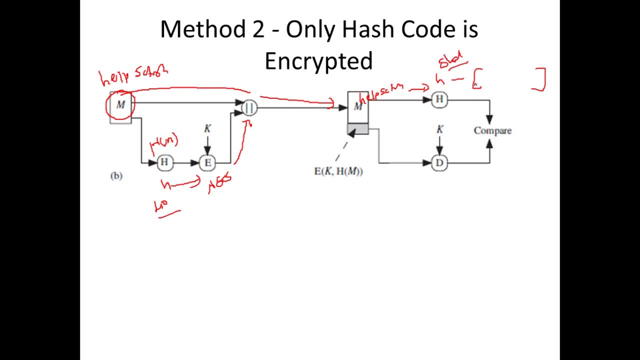 if he is going to use sha one hash function and this 40 digits are hexadecimal characters and he is also having this encrypted hash code coming here. so this is an encrypted hash code that's been sent and they are going to take this encrypted hash code and decrypt it because this 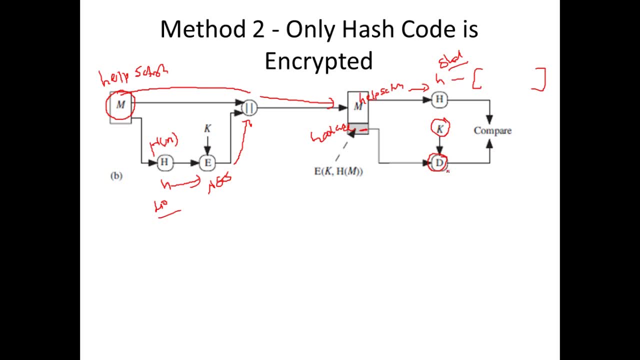 is encrypted. right, we'll decrypt it using a key and this hash code will be compared to the generated hash code. if both of them match, then we can say we have received the file just like what it has been sent. so this is method two. only we are encrypting hash code here. what is the advantage of this? 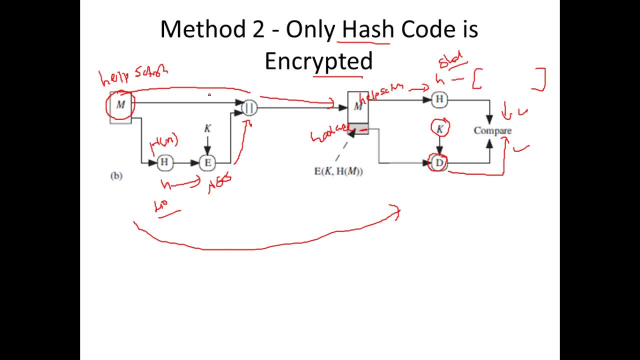 the advantage is, say, advanced encryption standard or any encryption standard takes a lot of time in going in for encryption right. so when we think that the message is not confidential, we just go with encryption, the encrypting the hash code alone, and the message is sent as plain text. 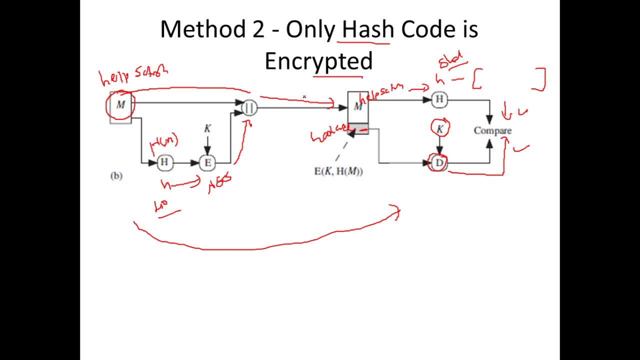 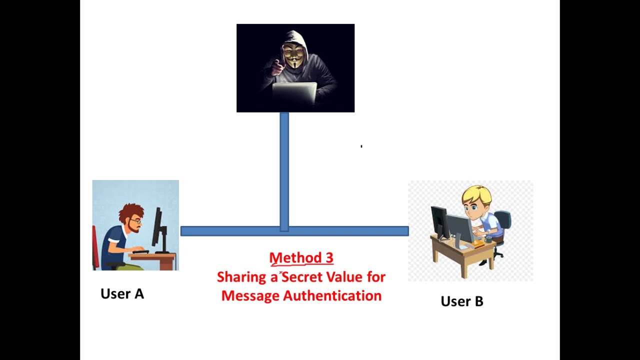 our main focus here is to ensure that the message is not halted during its transmission. we'll take a look at method three again. this method is different from method one and two. it's called sharing a secret value for message authentication. what is that? user a has a secret? 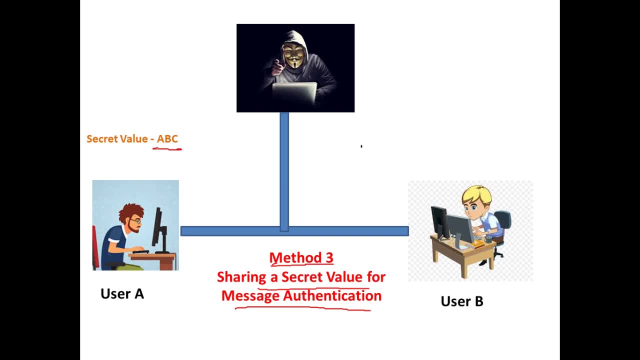 value that only e knows. it's only private to him say, the secret value is a, b, c and he shares that with his friend. so user b also knows that secret value. only these two guys know that secret value. and user a has some file in information he has to send, say, help, satish, is the file content? so what he's going to do is he's going. 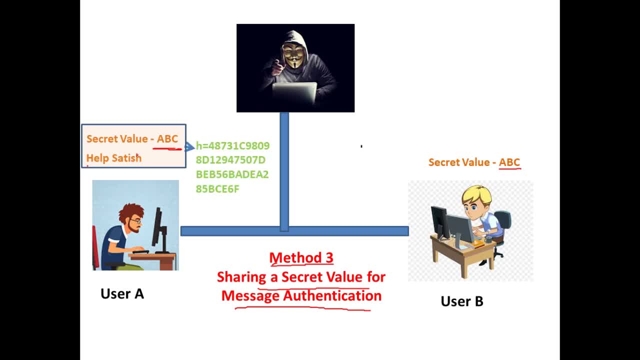 to take the secret value a, b, c. help. satish is going to hash it. so this entire thing will be given to this function h of m is going to get this 40 digit hexadecimal character. so all my hash functions- here i refer to sha1, which leads to 40 digit hexadecimal character. so this hash value is: 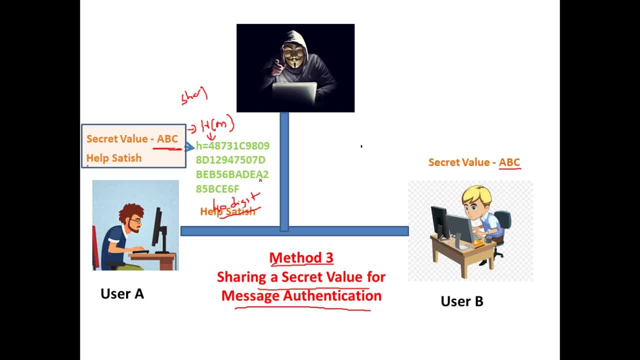 going to send it to his friend. that's the secret value of this function. so what he has to do is: he's okay, let me just erase this along. so this is hashed. what is this represents? this is an hash value corresponding to secret value plus the text. now, after getting this hash value, 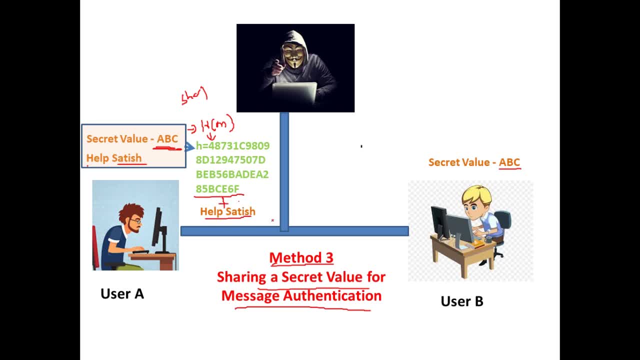 you will concatenate that with the text- help Satish, and you will be sending that to his friend. now his friend gets the hash value and this text. what he will do is he will take this plain text and he knows the secret value right. so using this plain text and secret value, you will generate a hash, so you will give. 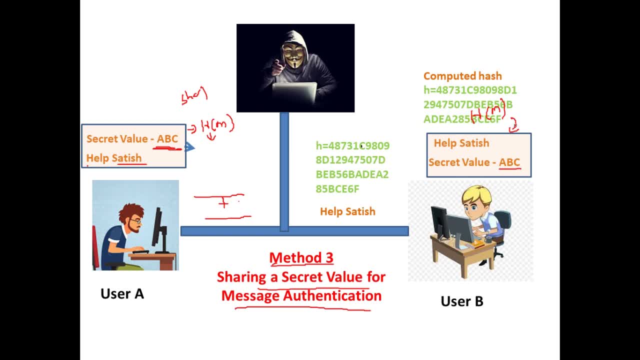 this to H of M: what is M here? these two things. and then he will compute and hash. so when he computes and hash each, you will compare that with the hash that he has received. so this is the computed hash, this is the received ash. only when they match you can say that. 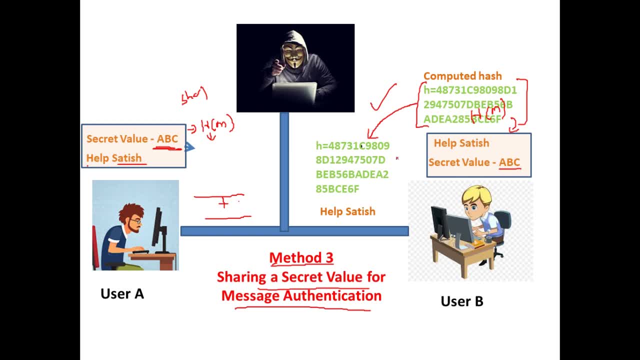 he has received the file the way it was sent. so what is the advantage here? this secret value is only known to these two users, and when they combine the secret value with the text, they'll be getting the same hash value, whereas this hacker doesn't know the secret value. so there is no way for him to, even if he alters. 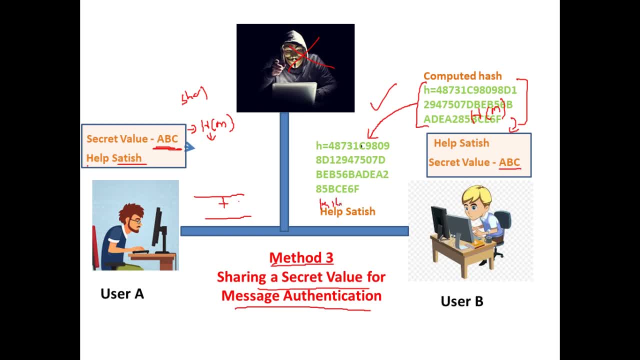 say, if he just alters some value here, if he enters, kill Satish and he sends a message and this guy is going to get the hash value and this guy is going to get the message. so what will be the message? kill Satish plus this ABC, he will. 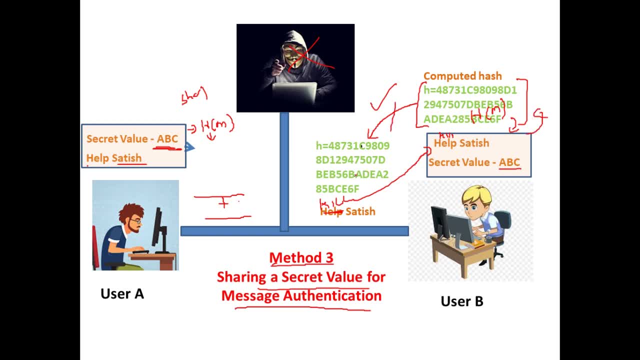 generate an hash, but this hash will not be equal to the received hash because this hash was computed as like this: secret values ABC, and the message is: help Satish. a secret value plays a key role. if somebody alters the text, it will be found out so again in your textbooks. this is the entire. 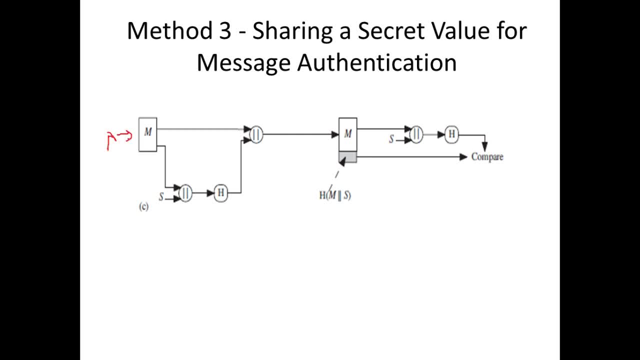 so you get this message from user a and what? what user a it does? he has a secret value s he concatenates this message with the secret value and then what he does. this is going to hash it. so secret value first message is hashed and then again is going to put this message and then this hashed value is going to. 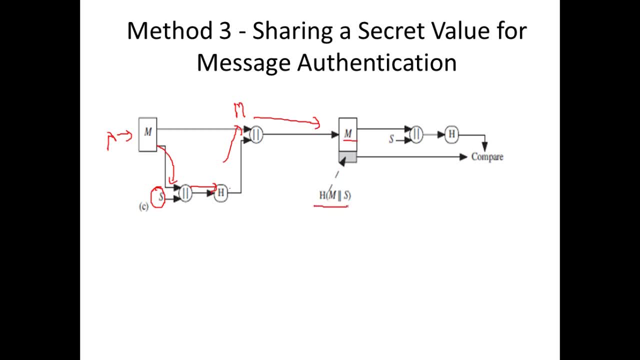 send it here. we are going to receive the message and then the hash value, so this message will be taken by user B E knows the value, and then you will combine the message with the secret value and then hash, and then you will compare whether this hash value is equal to the hash value is received when both these things match. 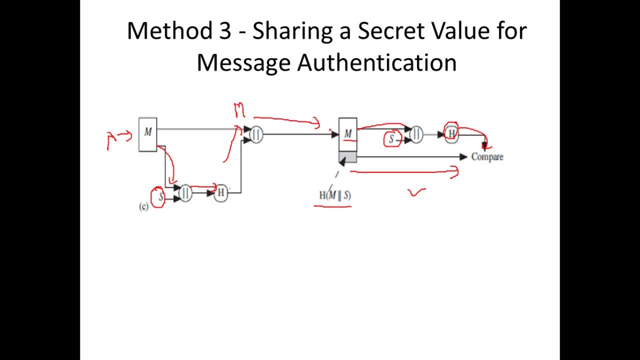 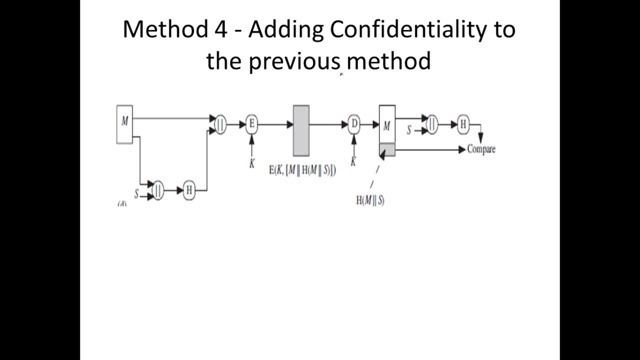 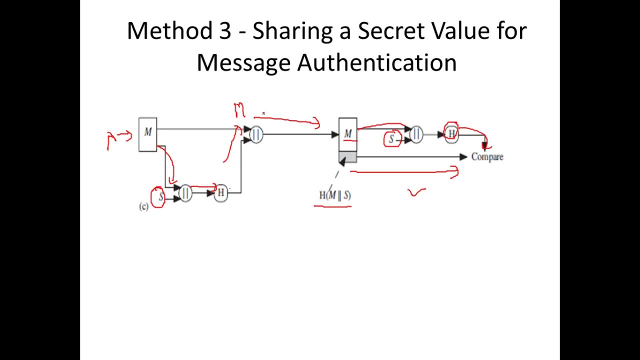 then we can say the message is authenticated. let's take a look at the next method, adding confidentiality to the previous method. this is method 4. this method varies from method 3 in a very slight. there's only a slight difference between method 3 and method 4. so again, let me repeat this: this is user a. he is sending this. 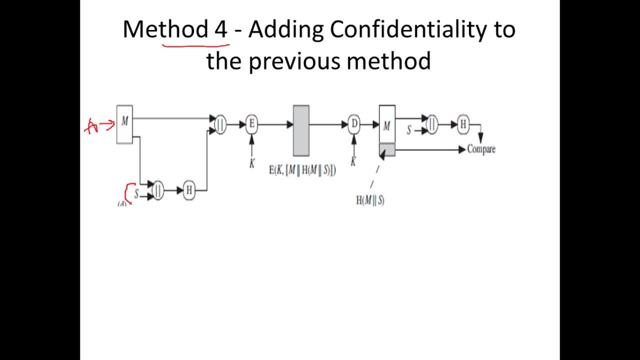 message m, and what he does is he has a secret value. he combines this message and secret value and hashes it to a 40 digit hexadecimal code and then he concatenates this with the message. so the message is satish, help satish. so he concatenates this 40 digit hash code with help satish. so this is the difference. he encrypts this. 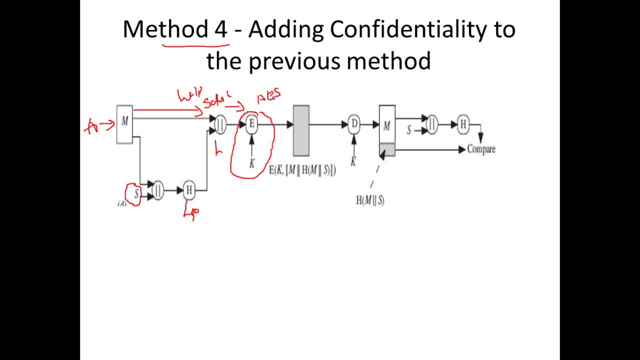 so again, encryption comes into place. he uses aes kind of an encryption and a key. and in what way it is different from the method 3 is the message is also encrypted. so we are adding more confidentiality to the previous method, and he sends it once. when you have an encryption you have to decrypt it first. 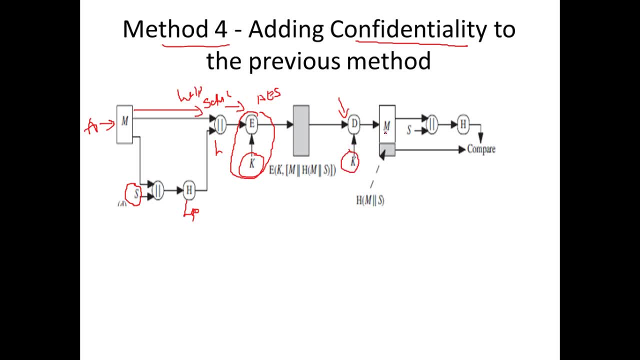 with the key and when you decrypt it, what you're going to get? you're going to get the message and the hash code. so he's going to take the message- he has the secret value- concatenate it and hash it. so this result is going to have- and he's received the message and the secret key- hashed value too. so 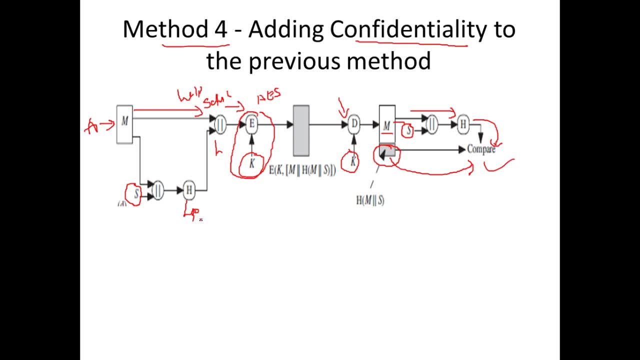 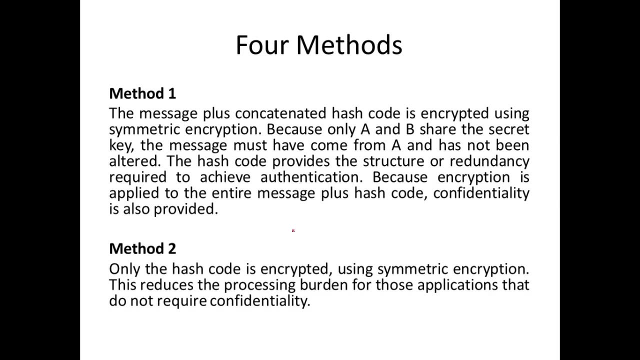 he is going to compare that. when both these things match, then we are going to say the message is authenticated. so i hope that is clear to you all. now let us go and take a look at the theory behind all these methods. i want you to go through the theory behind all these methods. 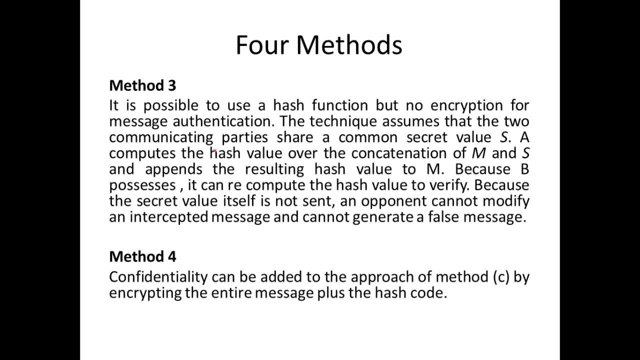 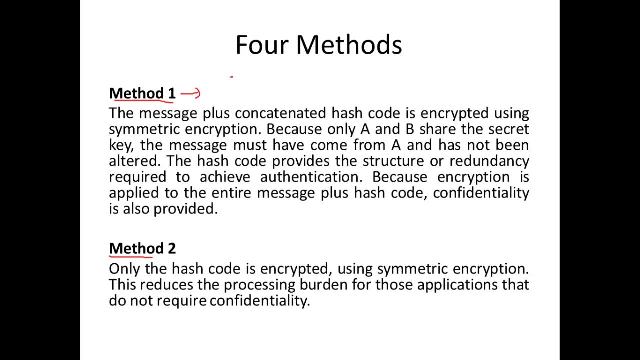 just in case, if you missed understanding that visualization, you can read through these paragraphs of theory. so when will you opt a method? when will you go in for any of these methods? say when you think the message, communication is important. say the message itself is confidential, if you think 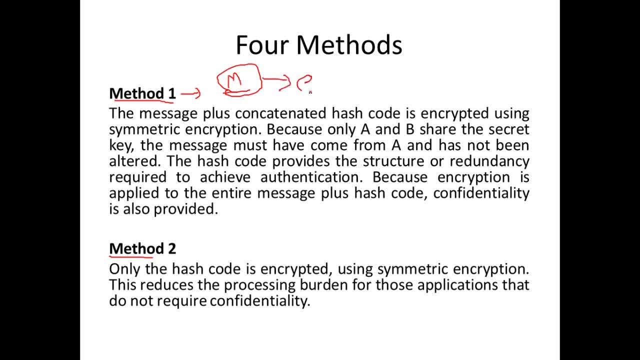 nobody should read your plain text message as such. you'll go in for methods that support encryption and decryption, so we'll encrypt and send. if you think the message is important, then you can read the message. if you think the message is not confidential, the only purpose is we have to check. 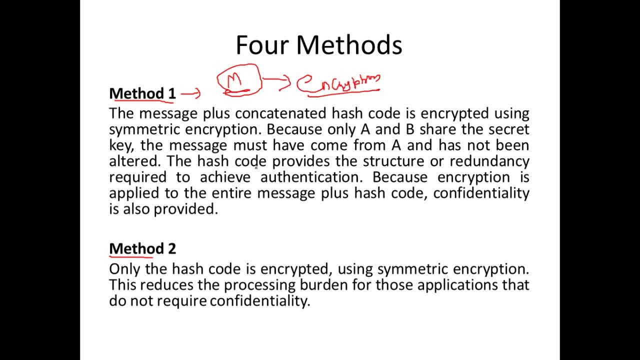 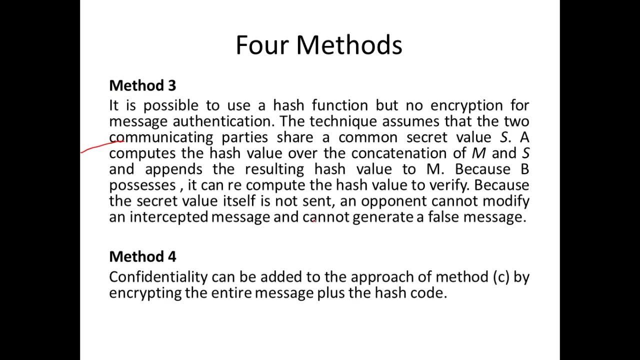 whether the authentication is fine. so here our message: confidentiality is not important. our only focus is it should be authenticated. then we can use method 2, wherein only the hash code is encrypted and then sent message is sent as plain text. if you are very much concerned about the secrecy, like 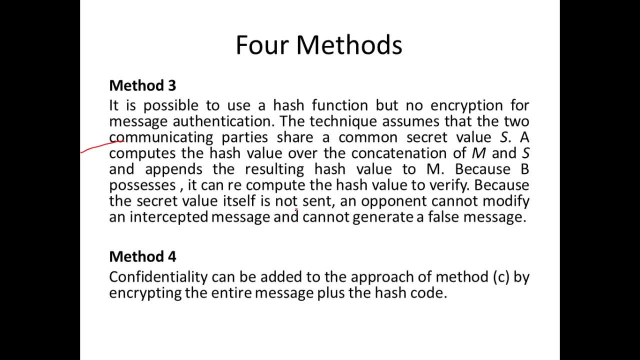 there's no way for an hacker to get hold of your message and alter it if you use a secret value. so you and the user who is receiving your message should share a secret value and then they can hash and send that secret value with the message. so the user will use the secret value. 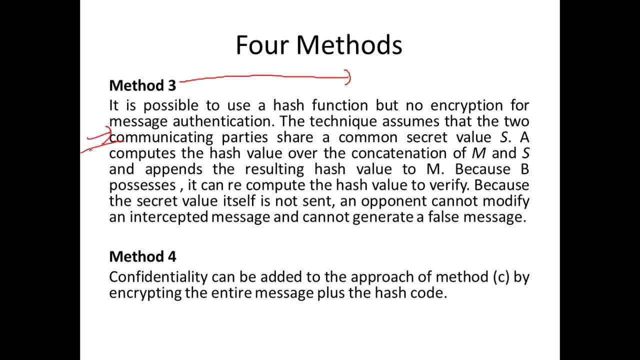 again, you will hash and check right. so this improves upon because we are having a secrecy here and method 4 is is adding more confidentiality to method 3. so it's like we'll be encrypting whatever we have hashed using our secret value and then we'll be sending it again in the receivers end. 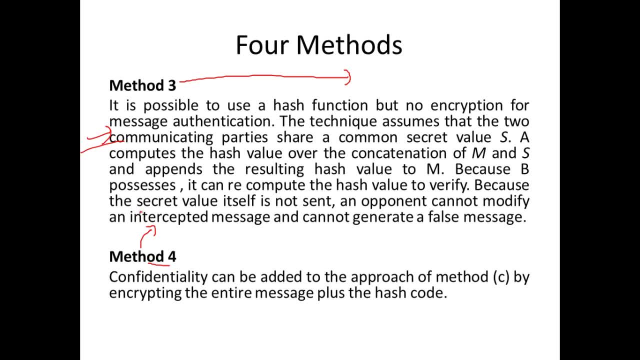 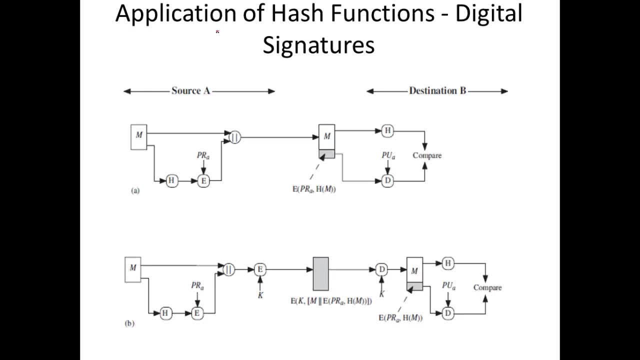 will be decrypted it. so that's how message authentication can be done using hash functions. now let us take a look at the next application of hash functions: digital signatures. so we'll be learning an algorithm on digital signatures- again an algorithm on message authentication using hash functions in detail, but these are just like an. 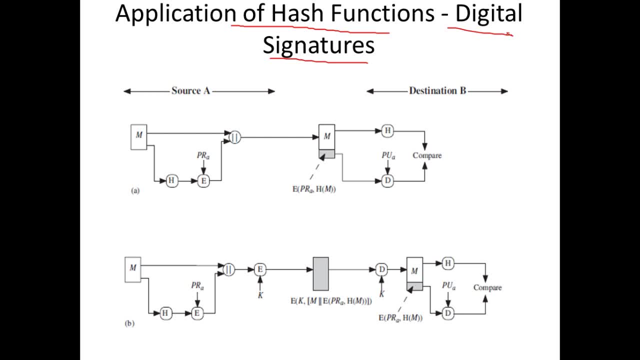 overview of application of hash functions. so what does that mean? what is the digital signature? so that's what i told you. if there is an user a, user a is sending a file to user b. so how will you know that only user a is sending this info? how can you verify that this information or file that is being 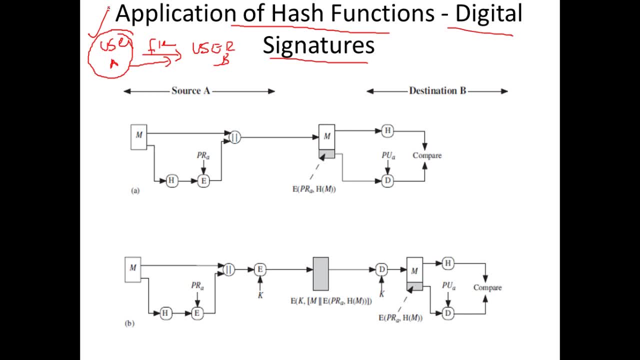 sent is only from user a, how can you verify the sender? so that's where digital signatures come into place, and we'll just take a brief overview of how digital signatures are used, all of a with hash functions in cryptography, so we'll go with this explanation here. so you have. 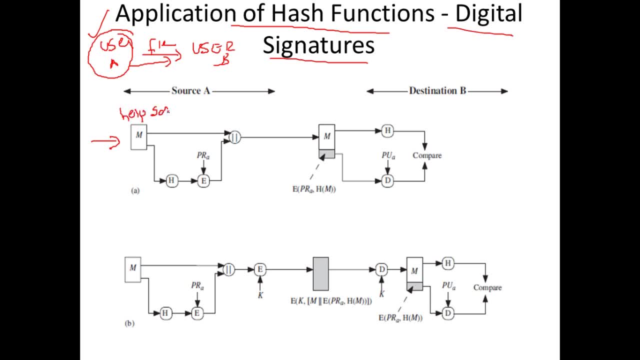 an user a message. always consider help satish to be the message. and what we are doing here is we are taking the message, we are generating the hash code. this is the 40-bit hash code or 40-digit hash code, and the 40-digit hash code is then encrypted, say in: 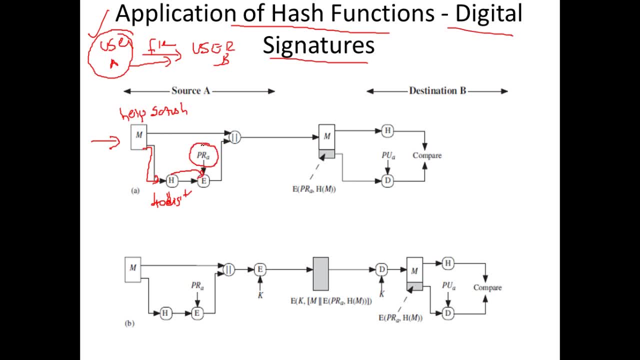 when you talk about encryption, we are using the private key of the user. so this user a, let's write. this user a has got two keys. one is a public key, another one is a private key. public key is known to everyone, it's open to all- whereas private key is very private to user a. 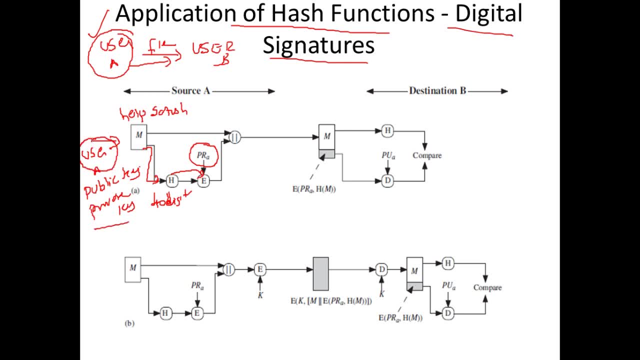 only user a knows private key. it's something like what we have learned in RSA, right, you have two keys: the public key is known to all, whereas private key is known only to the user. so this hash code is going to encrypt it using this private key and then is going: 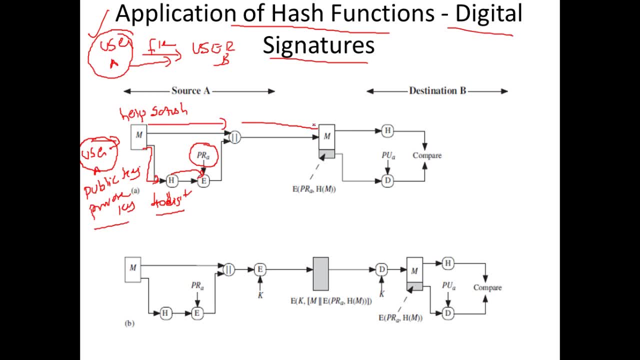 to concatenate this hash code with the message and then is going to transmit it. so here this message is sent as plain text, right? whereas this hash code is encrypted using the private key and sent. so what will be received? the message in plain text and the hash code that has been encrypted using the private key, and 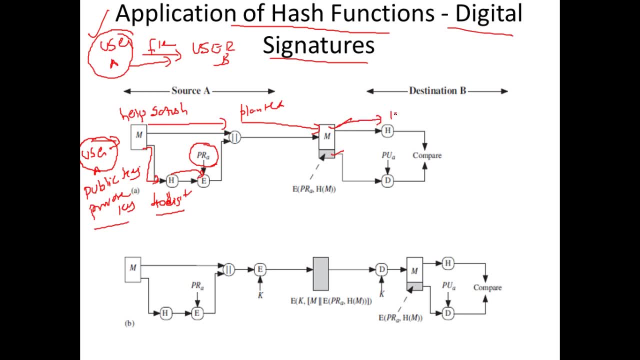 the message. the receiver will hash it again. you will send it to H of M and you'll get the hash value. so we'll get the hash value for the message, whereas here we are going to get this hash code right, that is encrypted. we will decrypt this encrypted hash code using the public key. 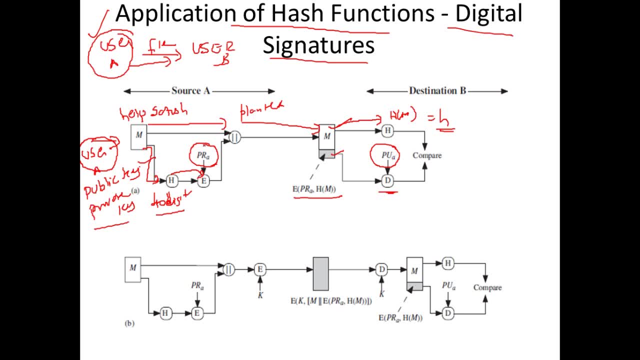 of user A, so you'll be able to decrypt it only using the public key of user A and one. when you decrypt it using the public key of usery, you will get the hash code. we compare these two hash codes. if they match, then the signature is verified. it. 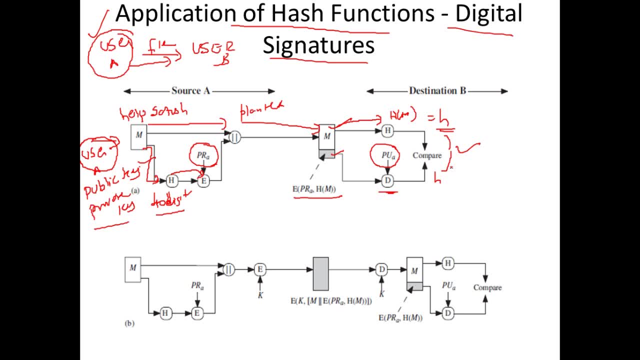 means that we have received this information only from the user who is intended to send this message. so what is the concept here? this private key is very much secure, right? it's only known to this user. so you can decrypt this hash code only when it is being encrypted by the private key of the. 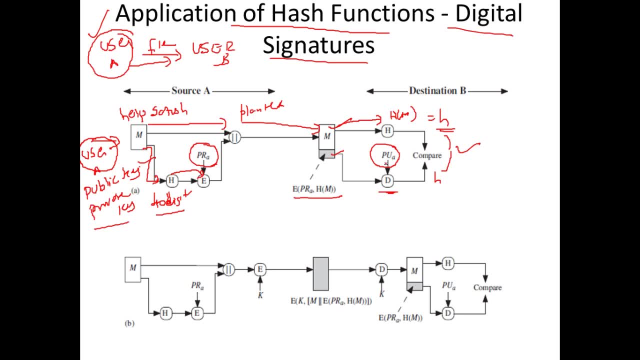 user so you can decrypt it using the public key one only when it is being encrypted by the private key of the user. that is the concept here, so that itself gives us the clue that the message that is being received is from this particular user. now there is a method to to that is it's it's adding. 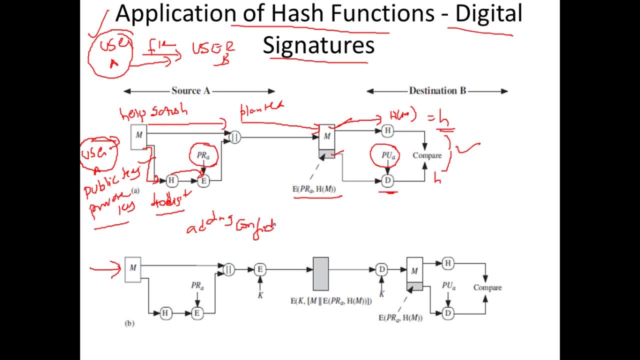 confidentiality. so it is ordering adding confidentiality here. what is that? in this method, the message is transmitted as plain text, only the hash code is encrypted using the private key of the user and being sent, whereas here we are adding confidence to confidentiality. that is, we are taking the message, hashing it, encrypting it, encrypting the hash code. 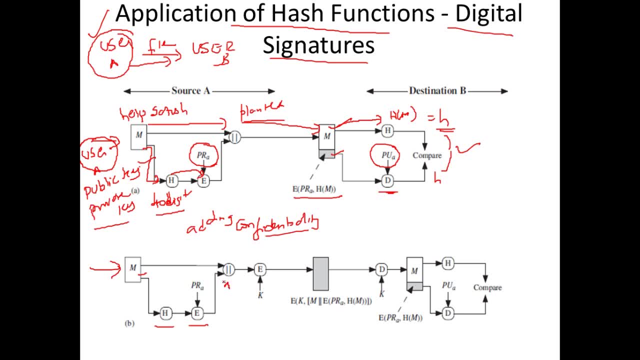 using the private key and we are concatenating this hash code with the message, and then this entire thing is encrypted. so this is adding confidentiality. so the message is not transmitted as plain text, it's also encrypted and sent. so once when you encrypt, you have to decrypt it first and after you decrypt. 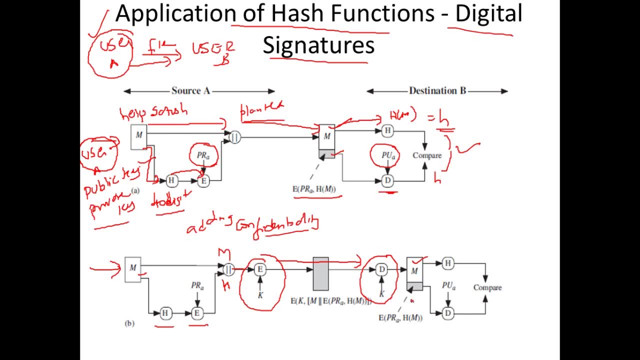 what all things you're going to have. you're going to have the message and the encrypted hash code. how can you decrypt this encrypted hash code? only using the public key of the user. so that is the key here. if a message is encrypted using private key, it can be decrypted only using the public key of the user and once. 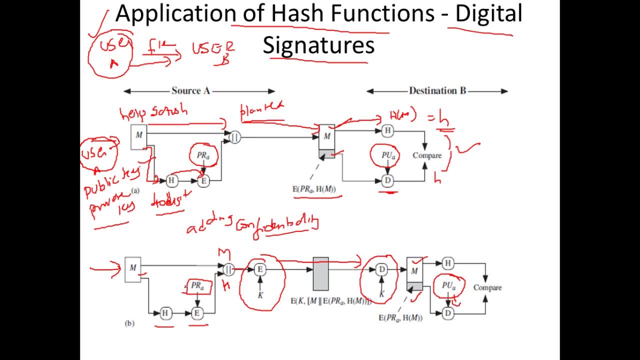 when you're able to decrypt this, it automatically means that this has been sent by this user and you're going to compare this hash that has been sent. by hashing this message right, you'll get an hasher. we'll compare these two things once. when they match, we say the user is verified. we can very well say the user. 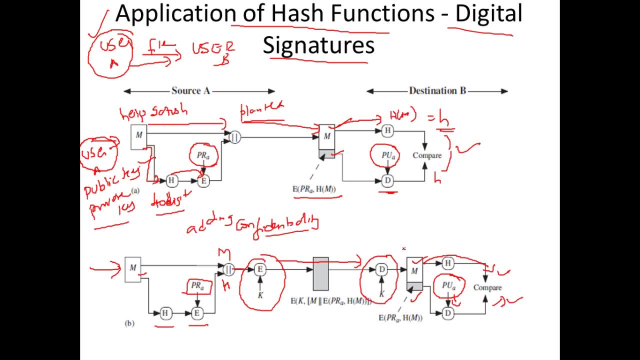 the file or the message that you have received is only from the user from whom we have to receive. so this is a very brief, a simple overview of digital signatures and how hash functions are used within digital digital signatures. in the coming classes we'll be looking at a separate. 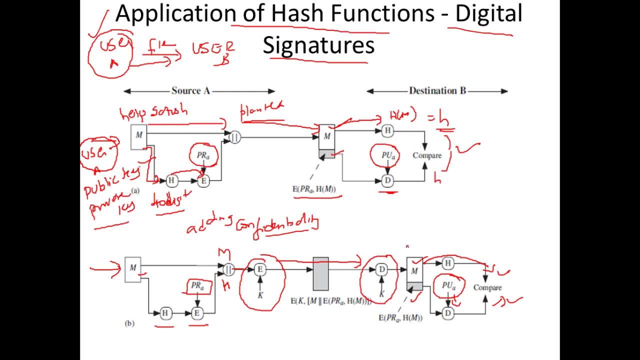 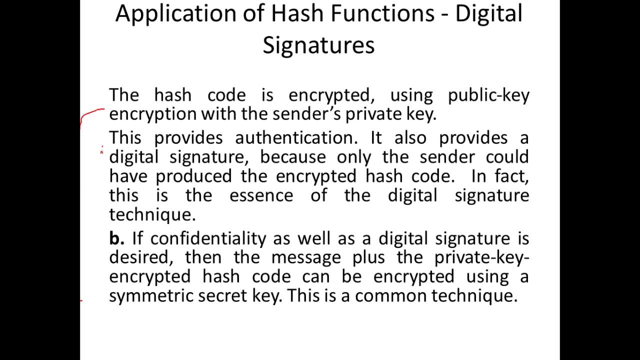 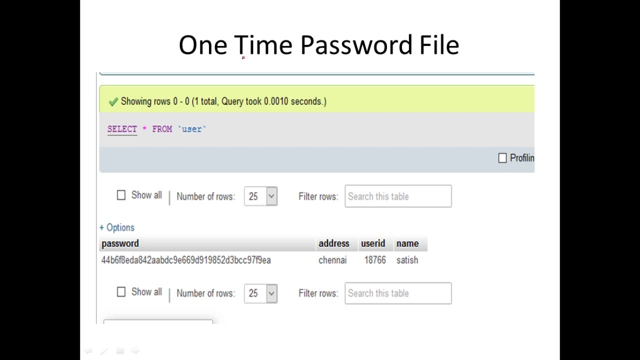 algorithm on hash functions and digital signatures too. so again, this is the theory with respect to digital signatures. you can very well go and read this theory. so we now take a look at another use of cryptographic hash functions, that is, cryptographic hash functions. that is a. it is used in securing passwords. let's take a look at how passwords are stored. 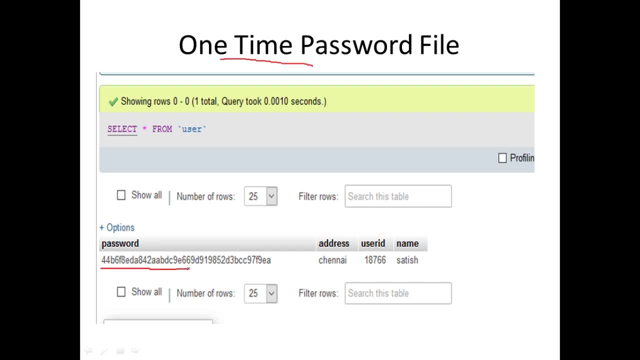 inside a database, the passwords are hashed and stored like this. so if an user's password is actually Satish, this is given to a hash function and it is hashed to a 40-bit hexadecimal character. if you are using SHA-1, it's stored like this. so what is the benefit of this? see how actually. 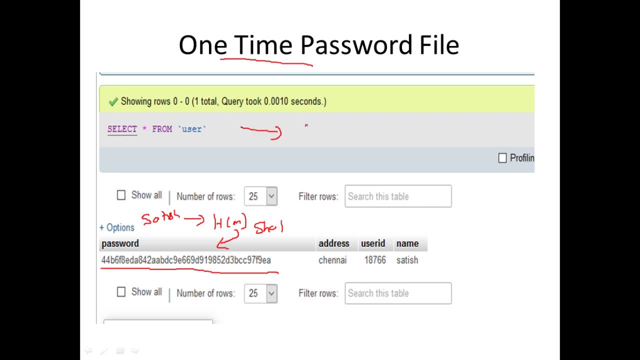 authentication happens here is whenever this user comes in, uses this form to enter his password, he will enter the password as Satish and this will be given to this hash function h of m, which will convert this to a 40-digit hash code, and this will compare. 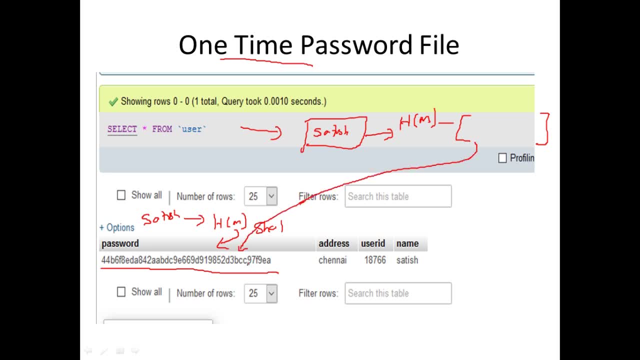 whether this 40-digit hash code matches the 40-digit hash code in the database. only when a match happens the user will be granted access. so how this is beneficial. for instance, say, a hacker somehow gets hold of a table, he gets hold of this password and from this 40-digits. 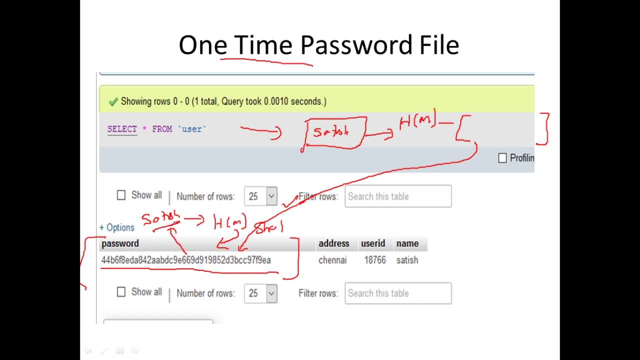 you'll not be able to go back and find. this password corresponds to this plain text, Satish. so once when he's not able to find, you'll not be able to access the system. say, he knows only this 40 digit right. so this 40-digit, if he enters as password, what will happen? 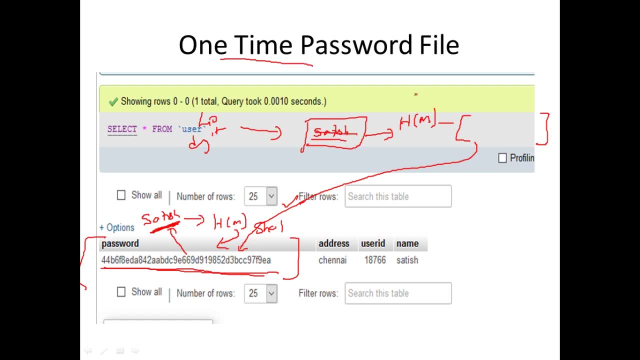 if he enters this 40-digit as password here, this will again go. so now our input is a 40-digit hash function, the next thing that we can do if we only have 40 digital digits here, what would happen? we will have to be able to find a password for this hash function. this is a well defined 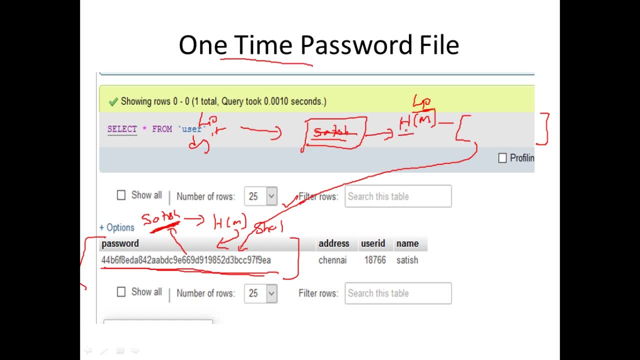 list of half digit hash function and password. this will be called a hash value, so this will also be like a definition of an already known password for some of our users. for example, value: again, this function will hash it. it will lead to a different 40 digits. so this hash value, 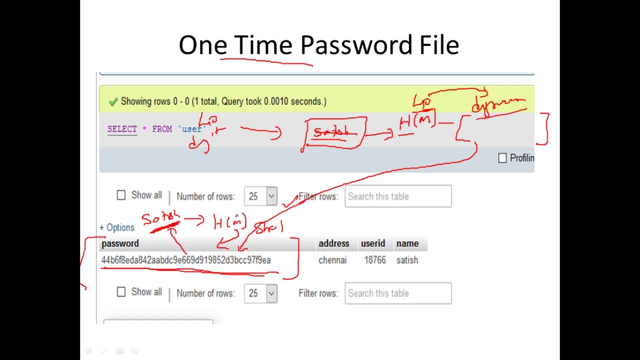 will be hashed to a different 40 digits, and this this will not match whatever that is existing in the database, so access will not be granted. so this is where the one-way feature of our hash functions is very helpful. even when a user gets the hash value in the database for the password, you will 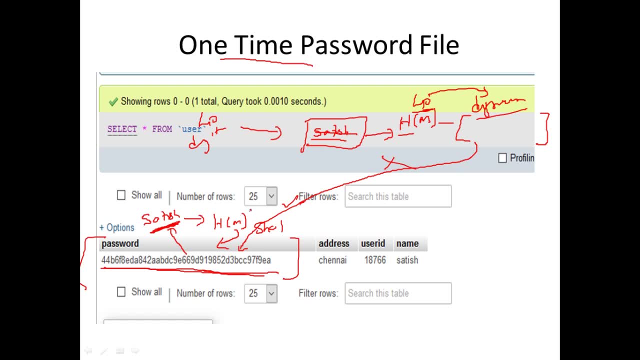 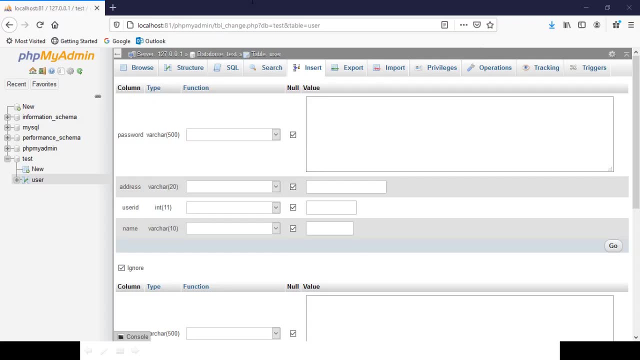 not get the password, so you can never access the database. and this kind of a feature is available in all the databases. now I'll just show you a demonstration on, on a php, my admin, a mysql database which I've installed here and you see here this is the structure of the table. I'll show you what is. 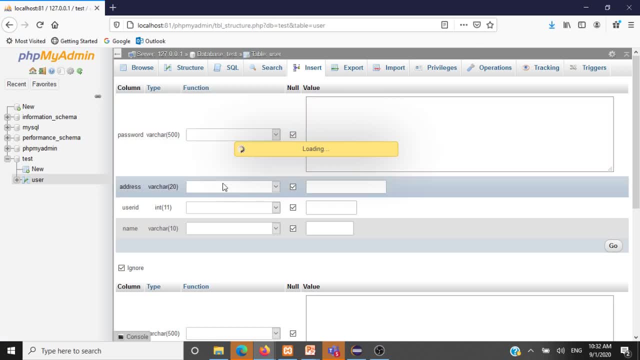 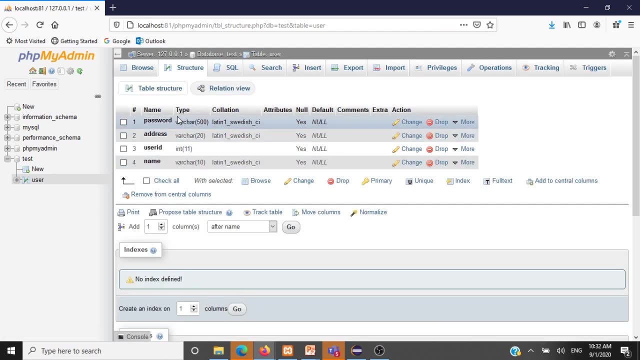 there they show you the structure just directly working with a database here. no problem if you didn't understand this, but just to tell you how it works. so this is the structure. it has a password address, user ID and name and if you want to use some kind of hostel to look at my example, if you. 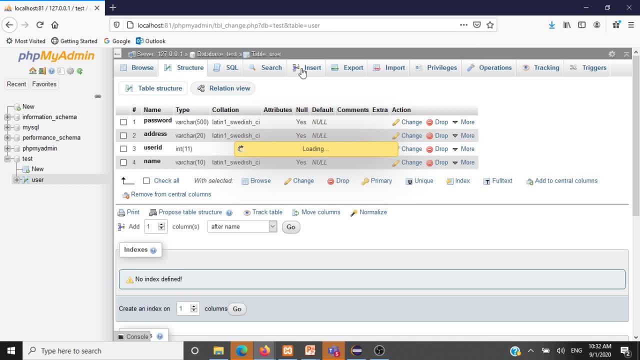 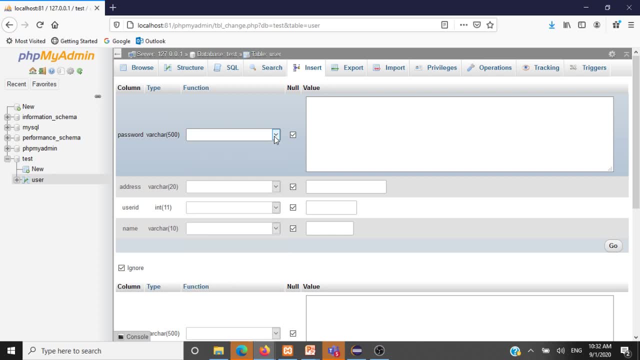 going to enter a password. what i will do. i'll go and insert directly. i'm inserting a password and here i can select the kind of security i have, say, and just go and select. i can either encrypt or i can go with uh hashing, say sha1. 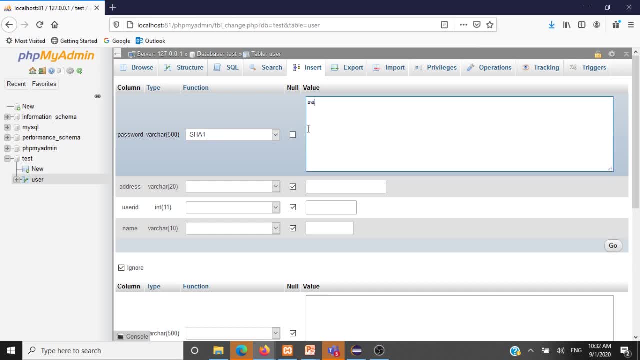 so whenever i store a password, say if my password is satish cj, so this is my password. but when it is getting stored in the database it will be hashed to a 40 digit exact decimal value and stored. so let me say address is uh pony and user id is uh 777. i'm just inserting a record here. 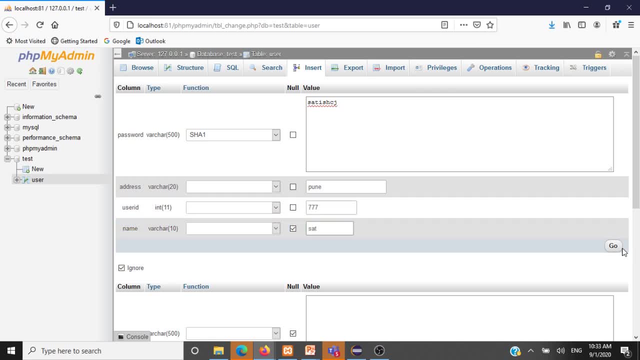 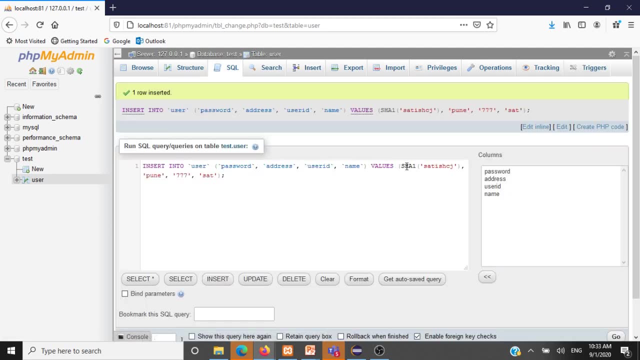 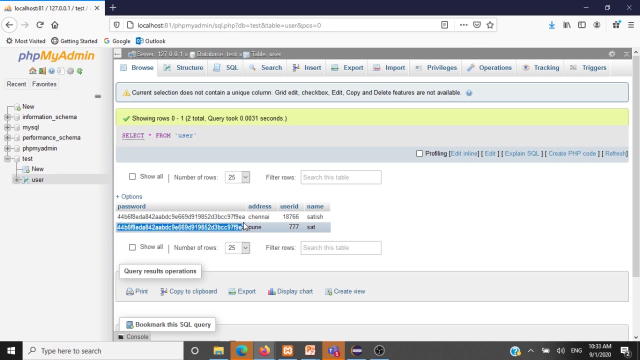 say, username is sat, and now when i give go? so what is the password i entered? satish cj is the password i entered. you see here it has been encrypted using this hash function. if you go and look at the uh data in my table, you can see it's not being stored as satish cj, it is being stored as a 40 bit. 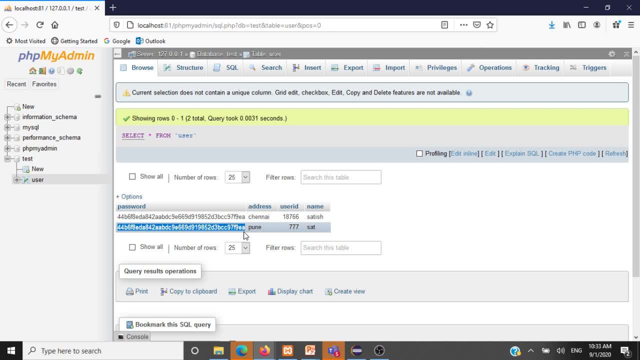 uh, 40 digit exact decimal hash value. so when an hacker gets hold of my database, you'll not be able to know my password because you'll not be able to get back satish from this hashed value. so this is where the cryptographic hash function should be. one way. it's very important. 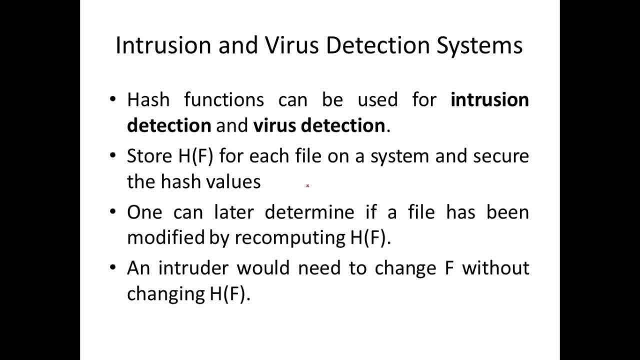 to understand the function of the hash function. another uh important use of uh cryptographic hash functions is in intrusion virus detection systems. say you are, you have all your system files right. what you're going to do is you're going to hash them and store them in some place. 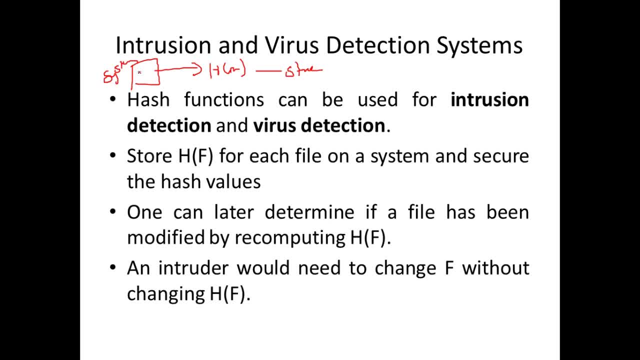 so if, if you want to check whether any malware, spyware or anyone, any virus has really altered your files, what you can do is you can, you can again take the files, pass it to an hash function and then you will get this hash value right. if you have to check this. 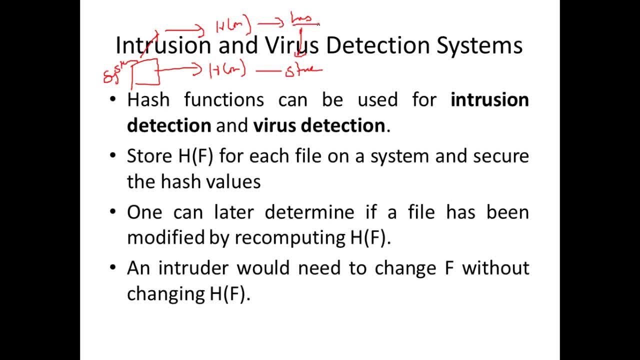 hash value with the previous hash value. so if there are any changes to this hash value, it means that somebody has altered your system files. if there are no changes, then your system is not being altered. so hash functions in cryptography are also used for intrusion and virus detection systems. 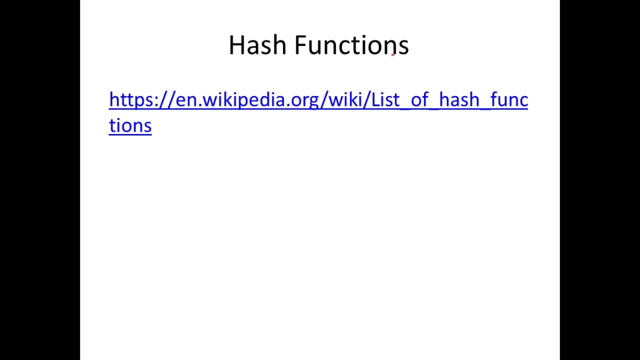 so you can go through a list of all the hash functions here. so we have a lot of hash functions. i told you about sha1. we have sha2. we have some six hash functions under sha2 itself. we have md5, md4- a lot of hash functions. so you can go and visit all the list of hash functions. 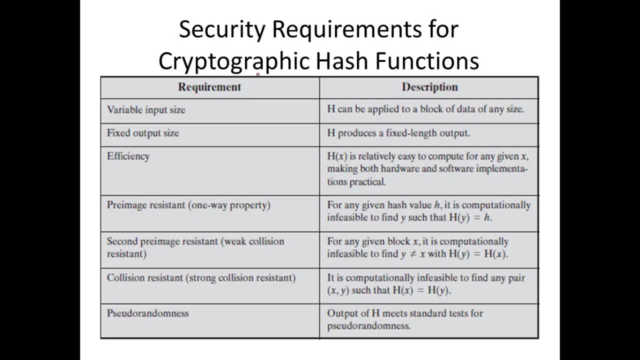 from this place. so we'll take a look at security requirements for cryptographic hash functions. when i'm going to use a hash function, what are the security requirements for these hash functions? it should allow variable input size. say, the message size that is given as input is variable length. that is one of the requirement. first message first. 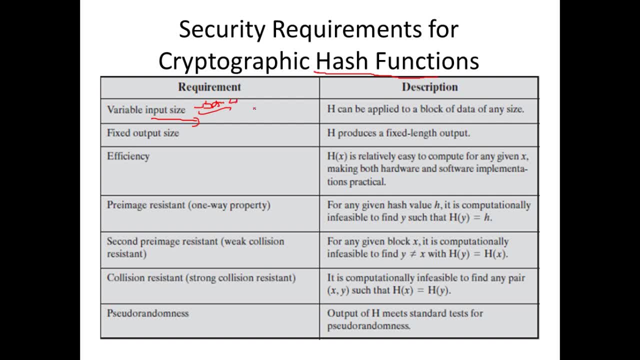 time i entered satish cj. the next time i enter. satish is not a good professor, so variable length input messages should be allowed, whereas the output size should be fixed. If I am going to use SHA-1, the output will always be 160 bits or 40 hexadecimal digits. 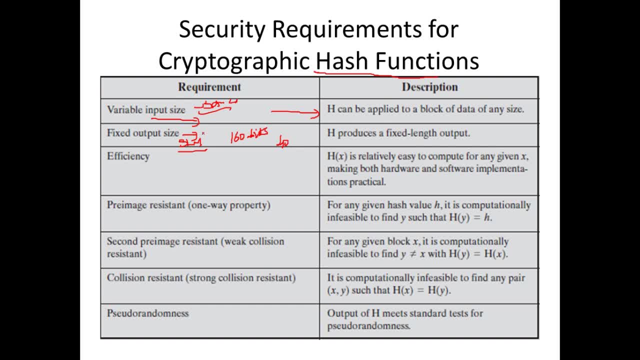 So if I am going to use this algorithm, then the output size should always be fixed, no matter what is your input size Efficiency. it should be very easy for us to calculate h of x, So it should not be like too much what to say. it should not make the implementation more difficult. 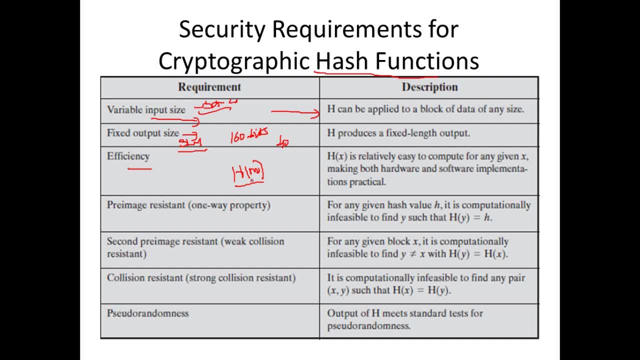 It should not utilize much of the resources. It should be relatively easy to compute h of x. That is again a requirement for cryptographic hash functions. We'll wind up looking at what is pre-image resistance and second pre-image resistance, What we mean by these things. 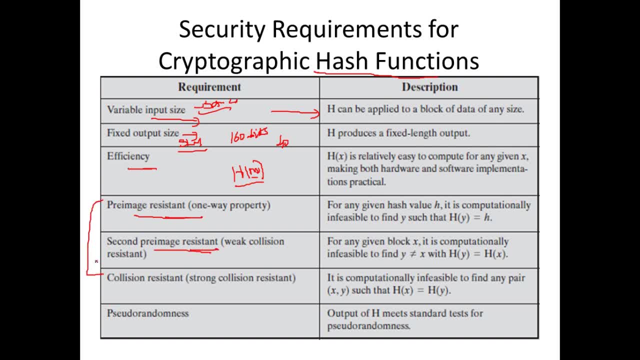 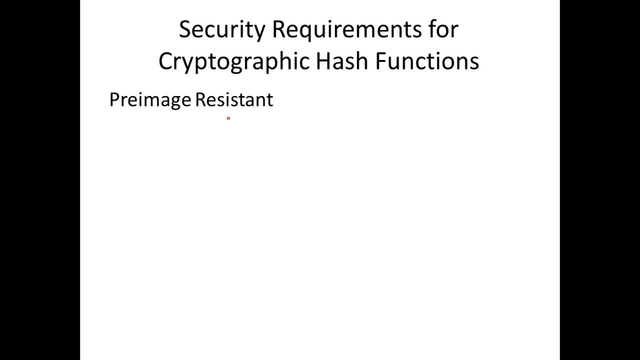 These are requirements. These are requirements for security, requirements for cryptographic hash functions. Let's take a look at that. What is pre-image resistant? So I'll just give you the meaning of this. Say: you are having this password, Satish, You are hashing it and storing it like this right. 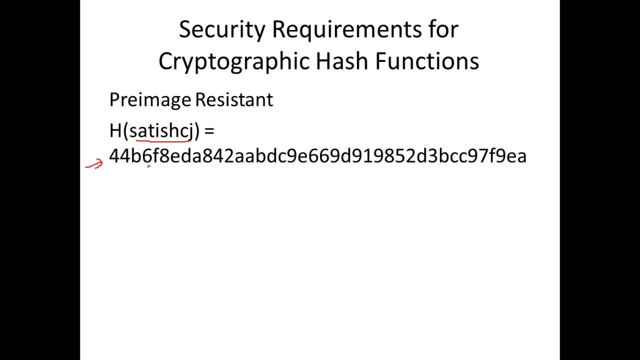 What do you mean by pre-image resistant? If this hash value, if this is being known to a hacker, no matter how hard this guy tries, he should not be able to get back the pre-image. So this value, Satish cj- is the pre-image of this hash value. 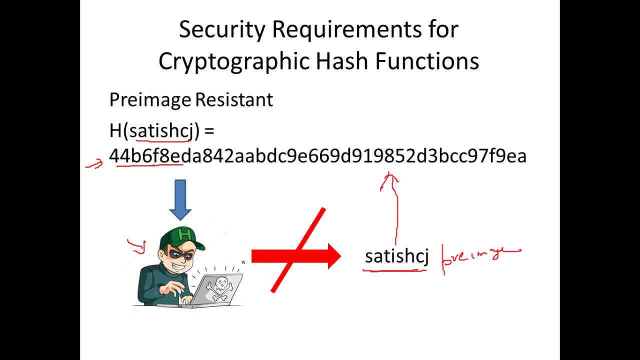 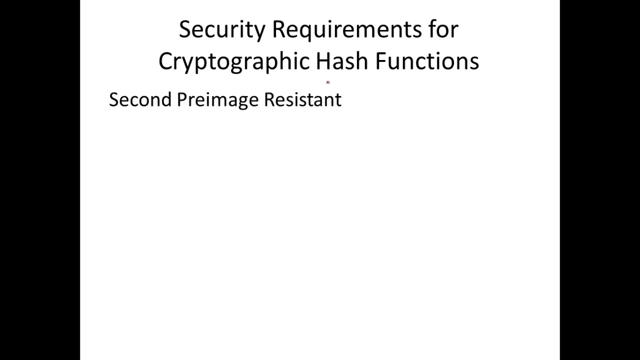 So when somebody knows the hash value, he should never be able to get the message. So that is called pre-image resistance. This is very, very important in cryptographic hash functions. The next thing is second pre-image resistant. What does this mean? 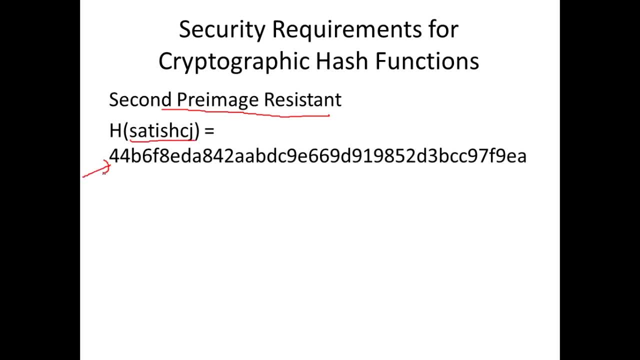 Say, if I have Satish cj is being hashed to this value, So what does that mean? If a hacker knows this is the corresponding hash value for Satish cj, you should never be able to find another input message m that will hash to the same value. 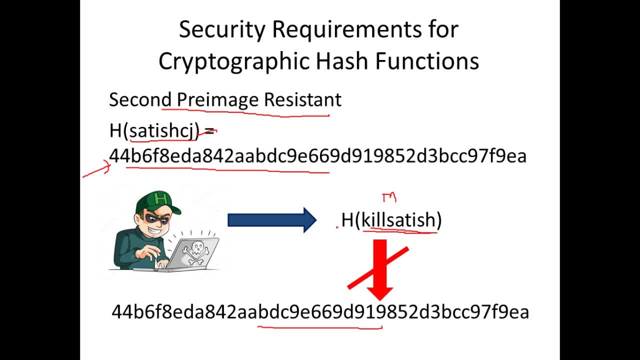 So this is a very important property. for instance, If Satish cj has sudah this hash value, The hacker should never be able to find another input message that will have the same hash value. So what is the advantage if he finds another input message with the same hash value? 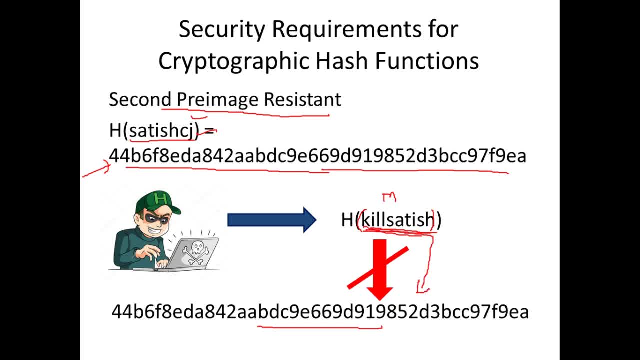 He can send this message plus this hash value as the original message to the user. Satish cj has just this hash value. So when this user has a message that will be sent to another button for the same value, says the drawer: Él toma una mensa original del hexado que�jae c Herren Y Times. this messenger should always be in a num summit so that to get this message the user can write himself as the original name. 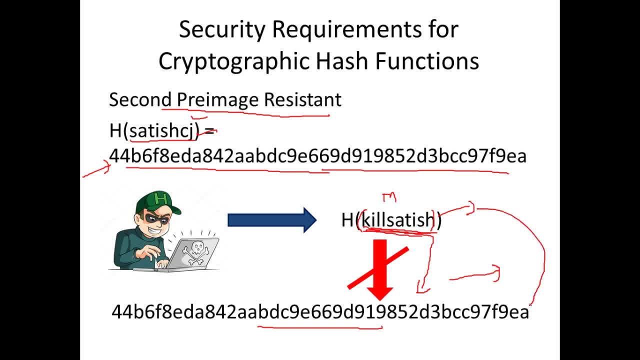 so when this user takes kill satish and he hashes it, you will get the original hash value, so you will think that this is the message sent by the user. so this is another very important property. that is, two different messages should not hash to the same value. in that case an hacker can.